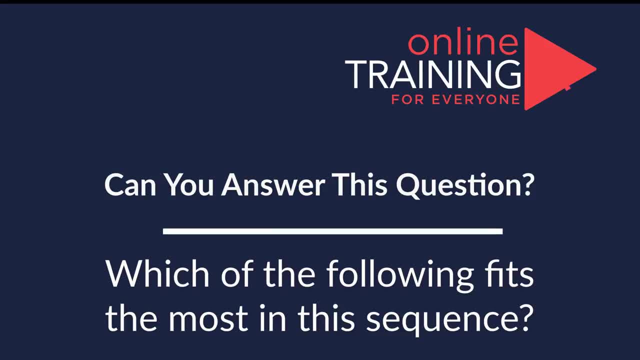 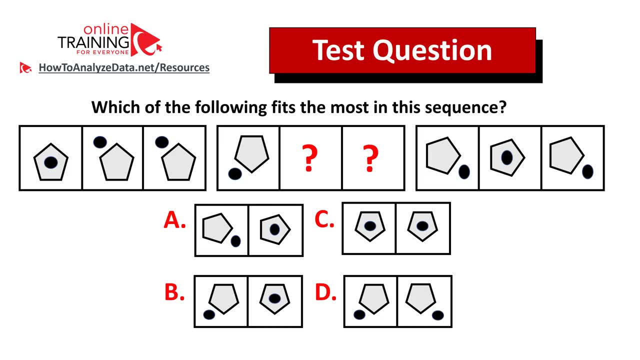 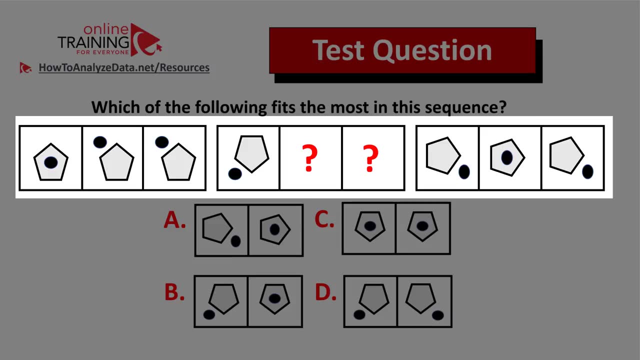 Let me share with you an interesting and tricky question which tests your pattern recognitions and logical reasoning skills. In the question you are presented with the three groups of shapes. The middle group has two shapes missing. All other groups have pentagon shapes present. 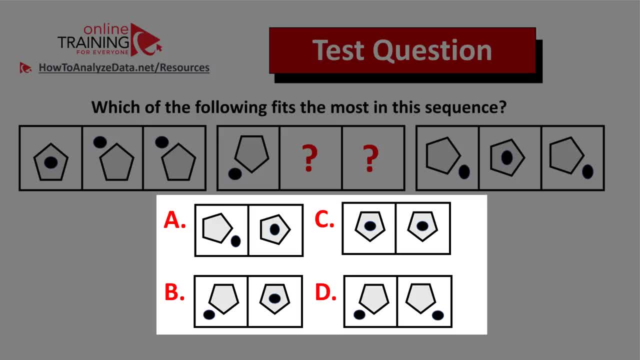 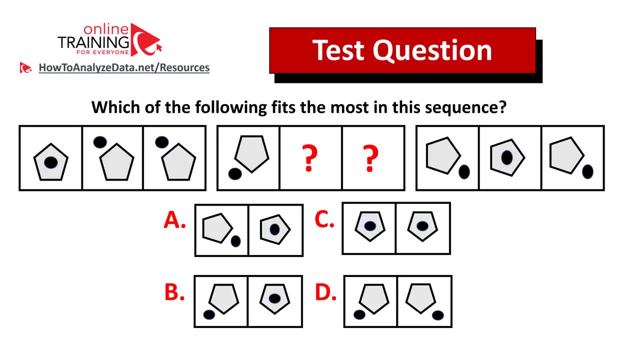 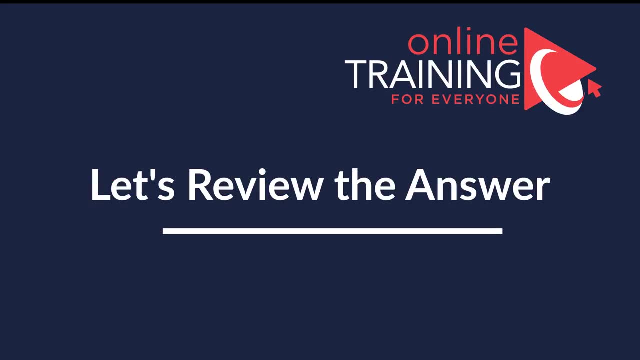 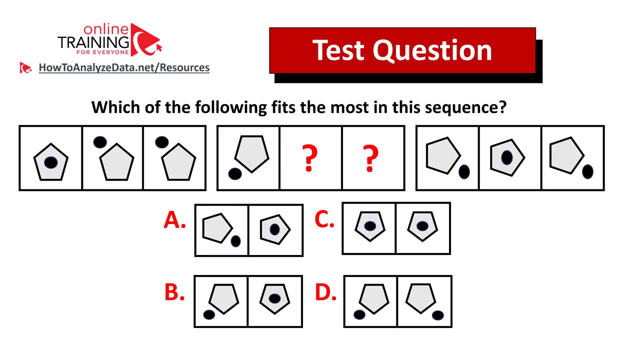 You have four different options to select the correct choice for the missing shapes. The choices are A, B, C and D. Give yourself 10 to 15 seconds to see if you can come up with the answer. Do you see the answer? Let's continue to see how we can solve this challenge and get to the correct solution together. 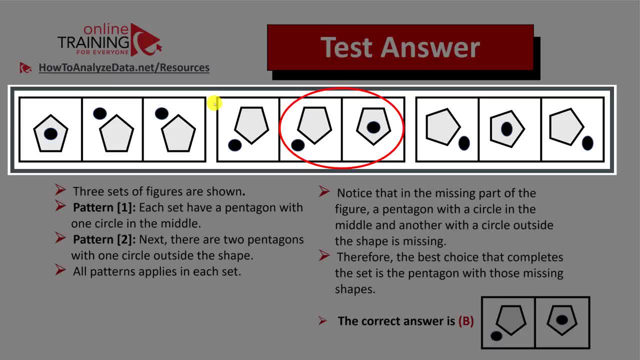 To solve this challenge, you need to understand patterns present in this question. There are two main patterns presented. The first pattern is the fact that pentagon contains the circle in the middle And the second fact is that two other pentagons in the group contain circles outside of the pentagon. 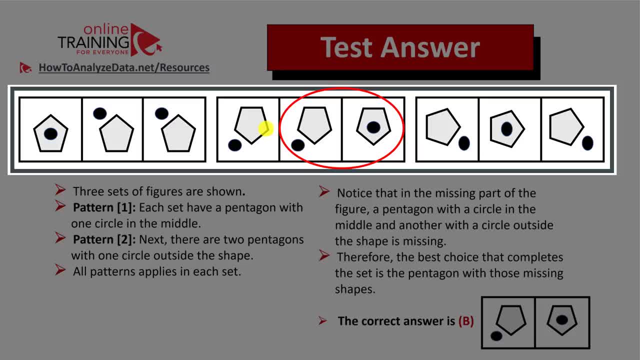 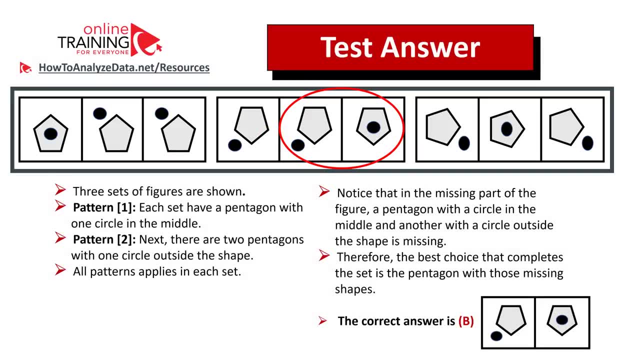 So to determine the correct answer, you need to look at the pentagon already present in the question. You see that the pentagon already present in the question has the circle outside of the pentagon, which means that the correct choice to answer this question would be two pentagons. 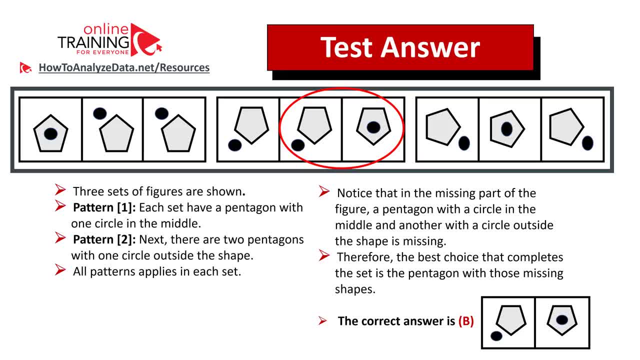 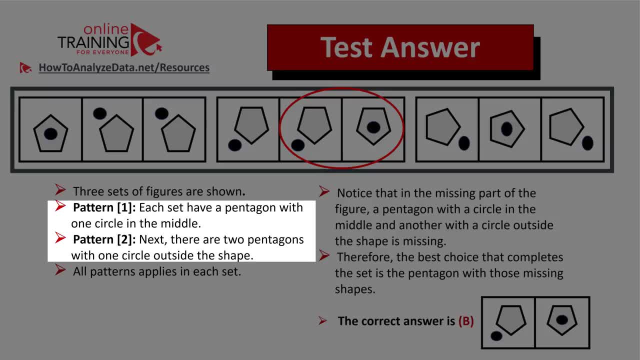 One pentagon with the circle outside And another pentagon with the circle inside. Let's recap: Always look for patterns, And there are two patterns present in this question. Pattern one is the fact that there is always a circle inside the pentagon. 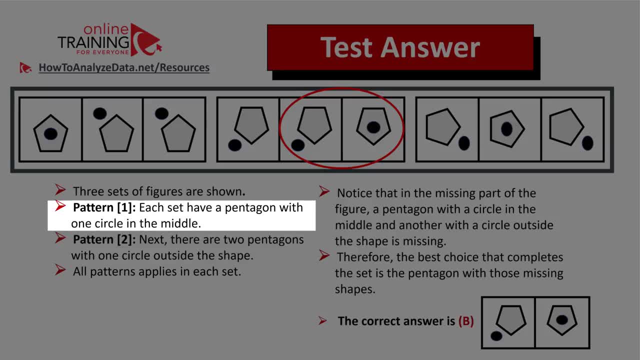 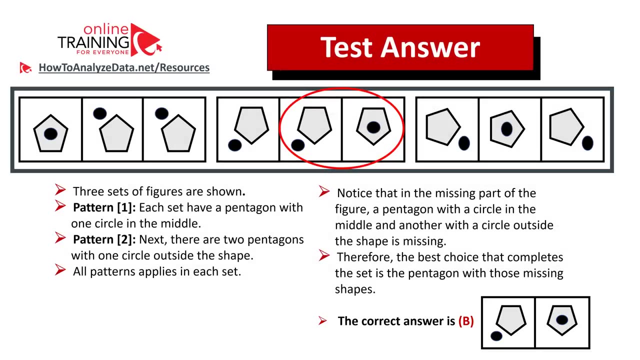 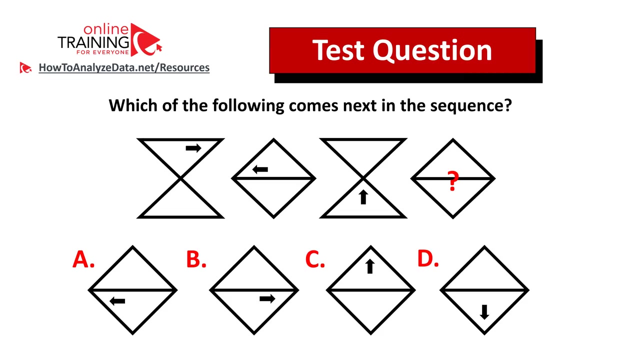 And pattern two is the fact that there are always two shapes with the circle outside of the pentagon. So the correct choice here is choice B. Hopefully you've nailed this question and now know how to answer similar questions in the test. Here is a very tricky question which is very unusual from the others. 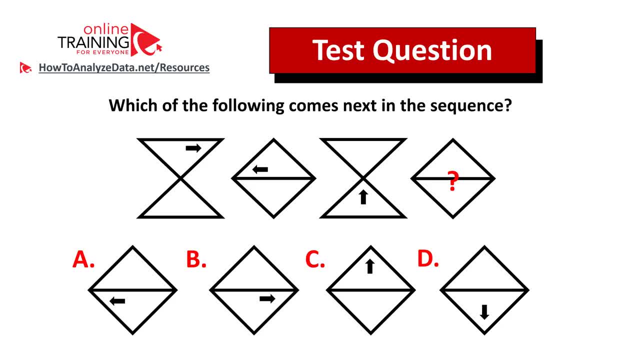 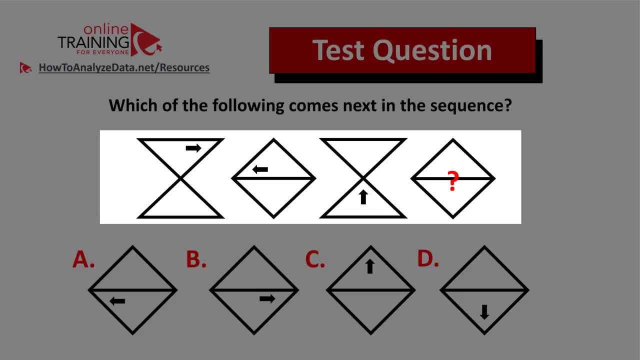 But once you know the pattern, it is very easy to solve it. Here is the question: Which of the following comes next in the sequence? You're presented with the sequence of four items And you need to determine the arrow's location for the item number four. 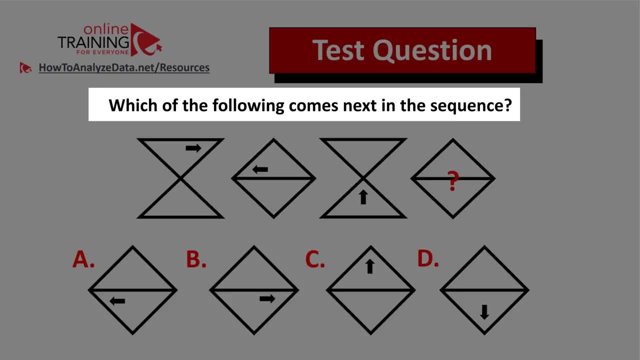 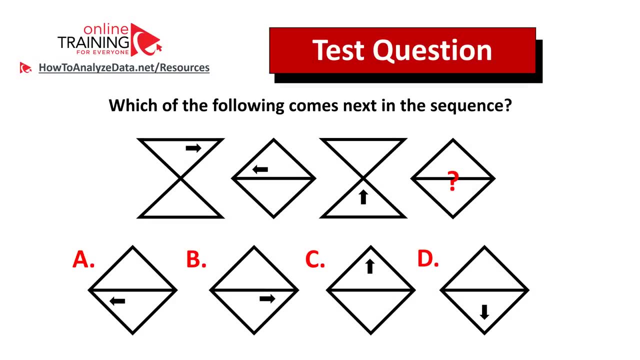 You have four different choices: A, B, C and D. Do you see the answer? The answer is not obvious. Let's try it. Let me tell you, But always look for patterns. Once you determine the pattern here, this question is very easy to answer. 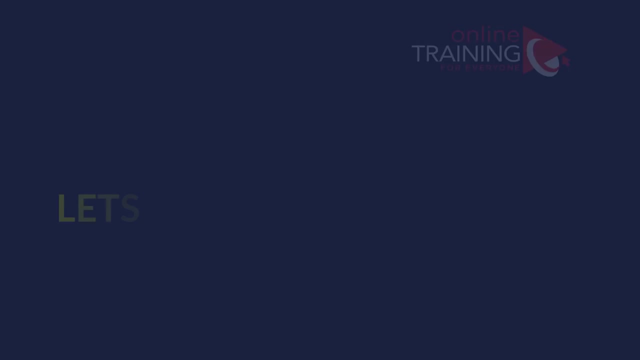 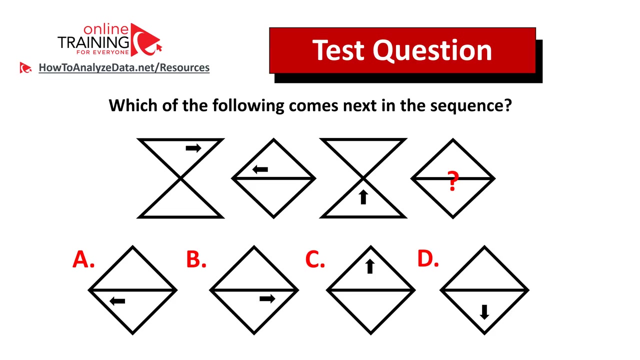 Give yourself 10 to 15 seconds to see if you can come up with the answer. Did you figure out the solution? Let's continue to see how we can solve this challenge and get to the correct solution together. As I mentioned, always look for patterns. 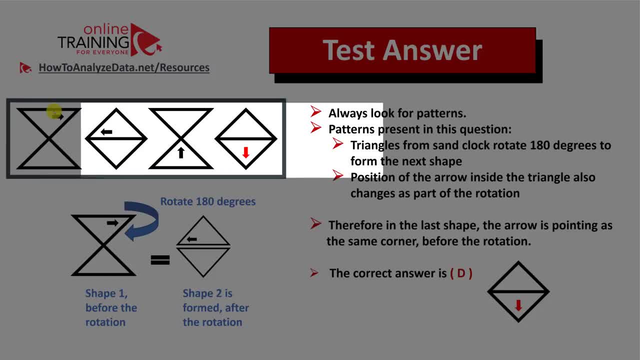 And the pattern here is triangles rotation. If we rotate triangles from the sandbox and we rotate them 180 degrees, we'll get to the square. And that's exactly what's happening between shape number one and shape number two, And this diagram below explains what's happening. 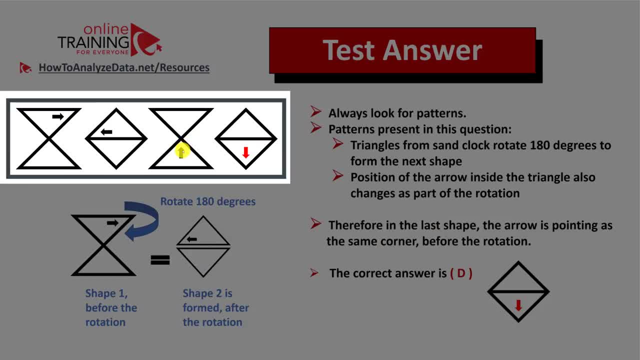 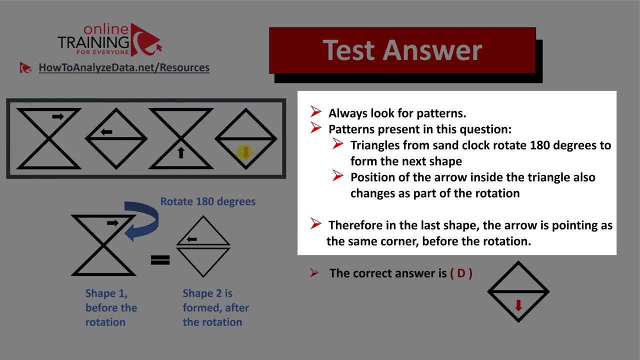 Once you figure out the pattern, you know exactly how to calculate the location of the arrow in the shape number four. Let's recap: Always look for patterns. Patterns presented in this question consists of two items: Triangles from the same clock rotate 180 degrees to the next shape. 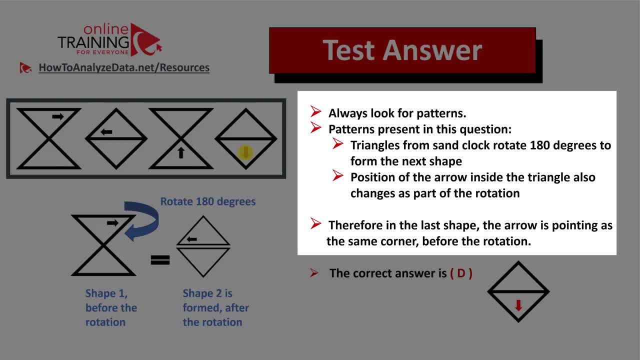 And position of the arrow is determined based on the rotation. This is why the next shape will be the one with the arrow pointing at the same corner as it was before the rotation. Hopefully you've nailed this question and now know what to look for on the real test. 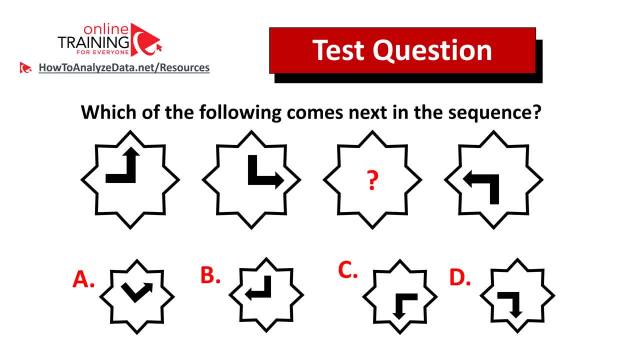 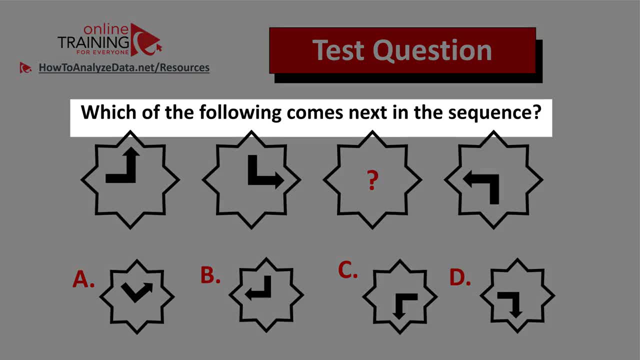 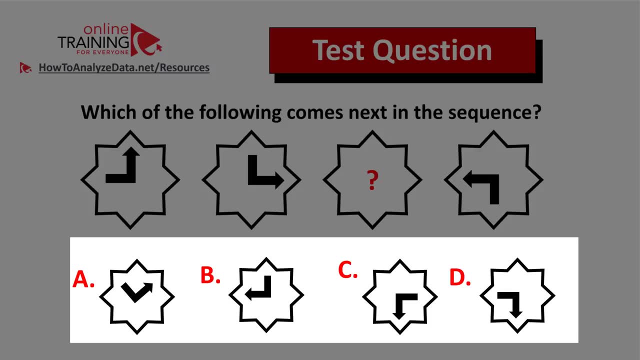 Here's the question from the test, But somehow I have a feeling that you might come up with the answer. Which of the following comes next in the sequence And you have a sequence of four shapes. The third shape is missing And you need to select the right shape out of four choices at the bottom. 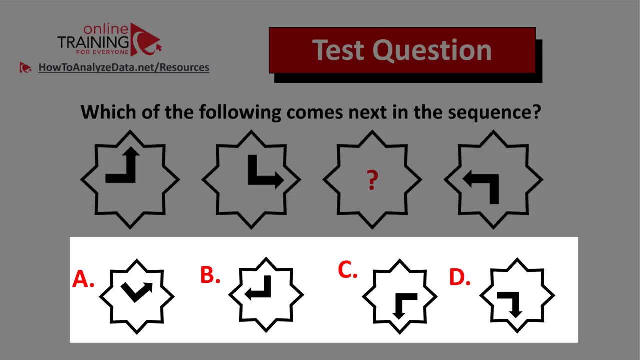 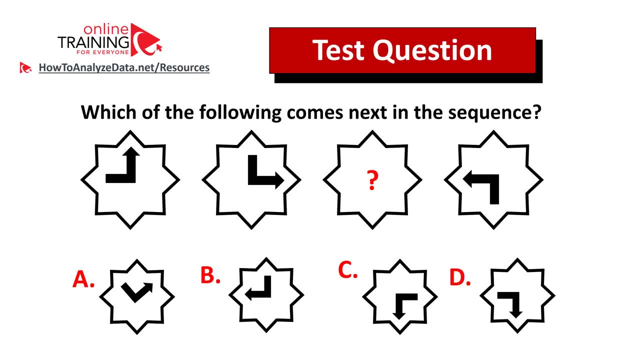 Choices A, B, C and D. Do you see the right answer? Please take a careful look to see if you can come up with the solution. Give yourself 10 to 15 seconds to see if you will get to the right answer. 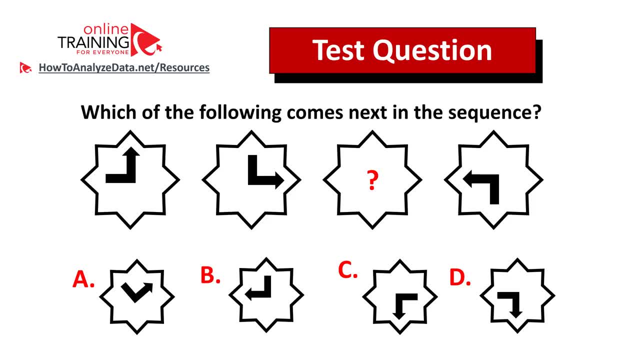 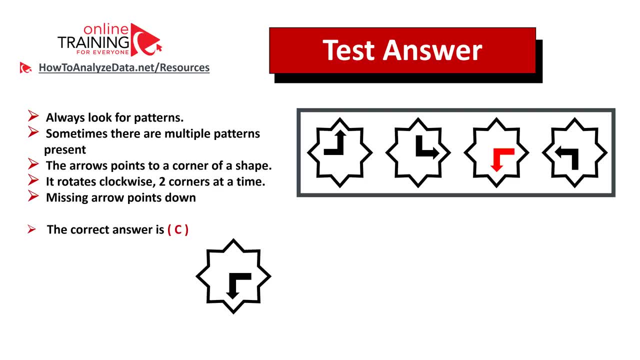 Do you see the answer? Let's continue to see how we can solve this challenge and get to the correct solution together, As usual. the answer might be a lot simpler than you think, But the key is to always look for patterns. So take a look at the patterns here with the shapes. 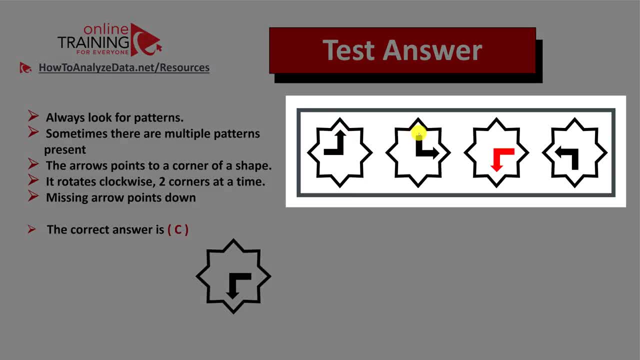 The first shape arrow points to 12 o'clock. Second shape points to 3 o'clock. You see that it clicked two positions between the first shape and the second shape. Then the next shape arrow supposedly will point to 6 o'clock, Because the last one points to 9 o'clock. 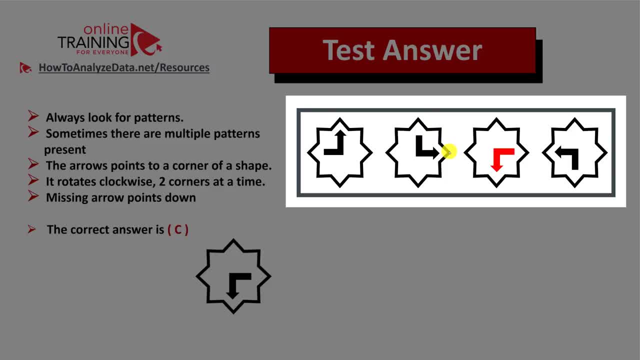 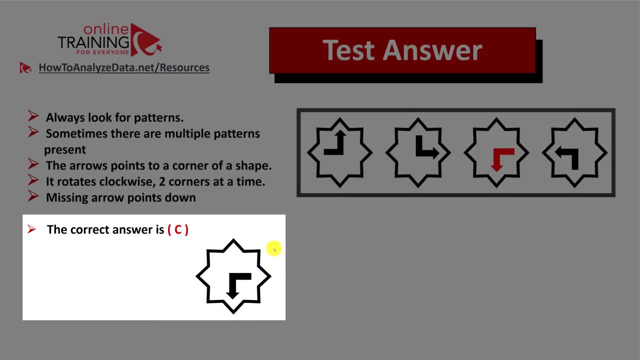 So that's the answer. You go two corners at a time and you calculate the next move using the formula. So the correct answer is choice D. arrow pointing to 6 o'clock. Hopefully you've nailed this question and now know how to answer similar problems on the test. 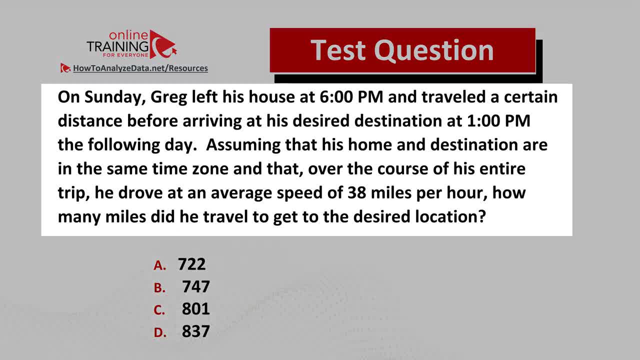 And now here's the question for you to try. On Sunday, Greg left his house at 6 pm and traveled a certain distance before arriving at his desired destination at 1 pm the following day, Assuming that his home and destination are in the same time zone. 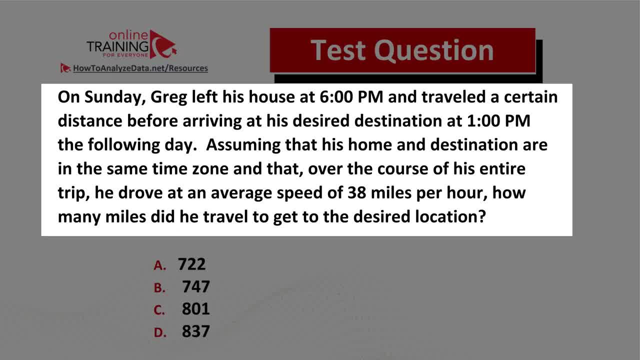 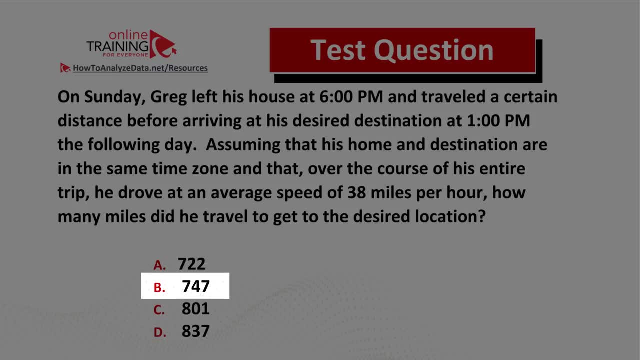 and that over the course of his entire trip, he drove at an average speed of 38 miles per hour. how many miles did he travel to get to his desired destination? And you have four choices to choose from. Choice A: 722.. Choice B: 747.. 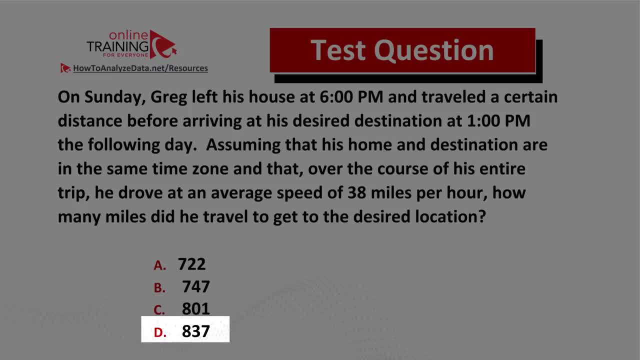 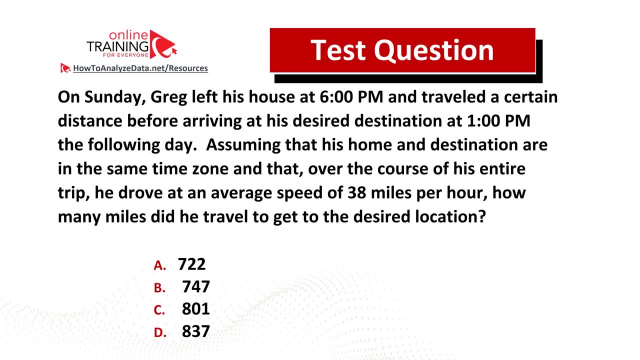 Choice C: 801.. And choice D: 837.. Do you think you know the answer? If you know the answer, please make sure to post it in the comments section of this video so I can give you my feedback. Thanks for participating and good luck. 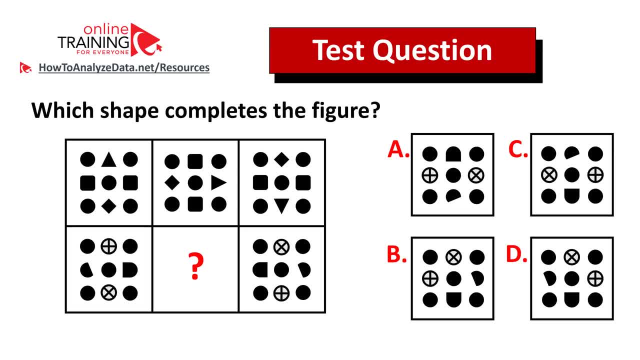 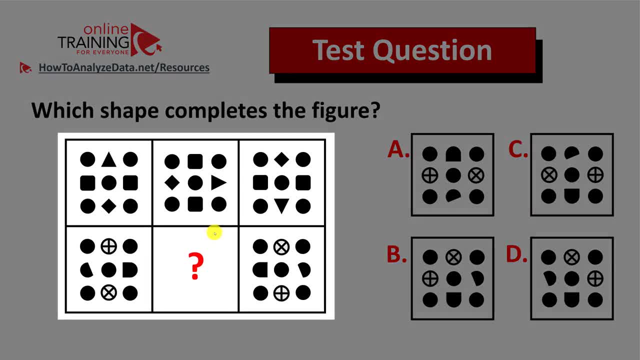 Let me share with you a tricky question which tests your pattern recognitions and logical reasoning skills. You're presented with a rectangle which, inside of it, contains six different shapes, and one of the shapes is missing. You need to determine which shapes completes the figure. 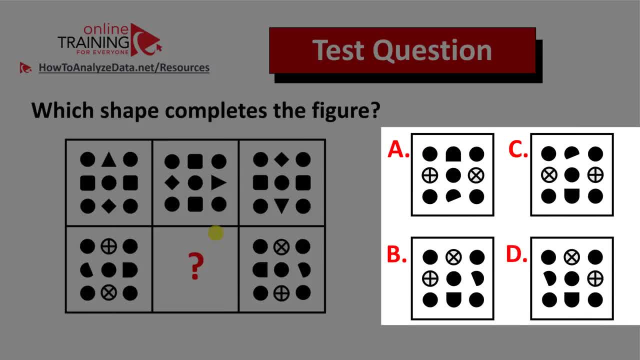 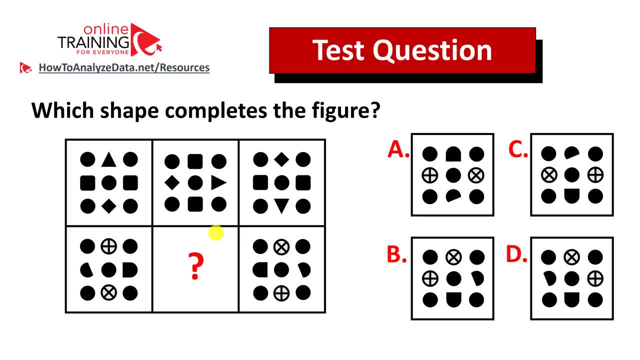 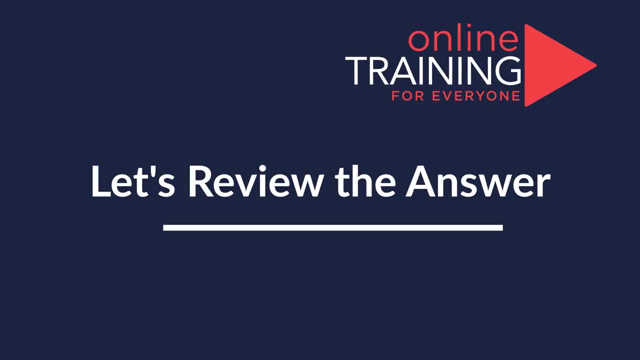 And you're presented with four different choices: Choices A, B, C and D. All of these choices look very similar. Now is the good time to pause this video to see if you can come up with the answer on your own. Did you figure out the solution? 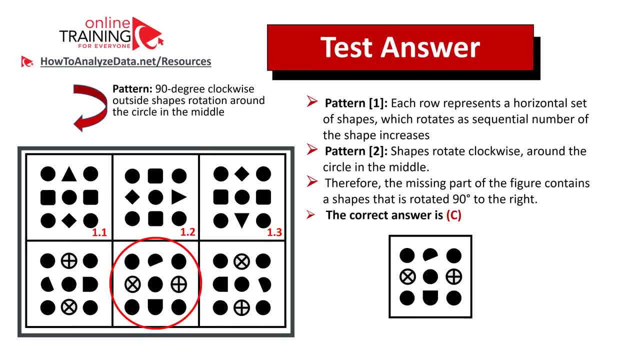 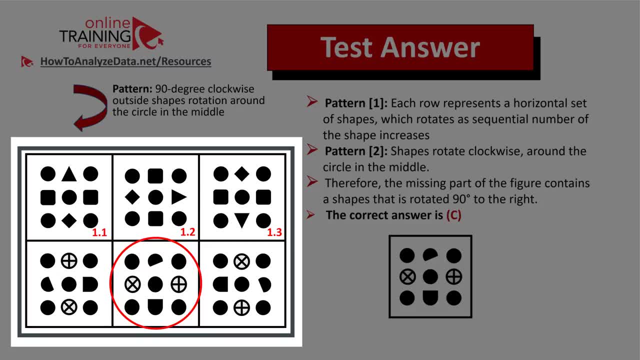 Let's continue to see how we can get to the correct solution together. As usual, my recommendation to you is always: look for patterns, And there are two different patterns presented here in this particular question. Let's look at the pattern 1.. Pattern 1 defines that the shapes go in the horizontal rows. 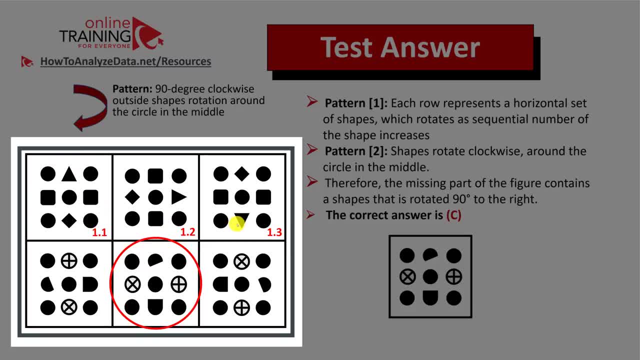 For example, this is the shape 1,, this is the shape 2, and this is the shape 3.. I grouped them as shape 1.1, meaning that the first one represents the first row, shape 1.. The next shape is first row, shape 2.. 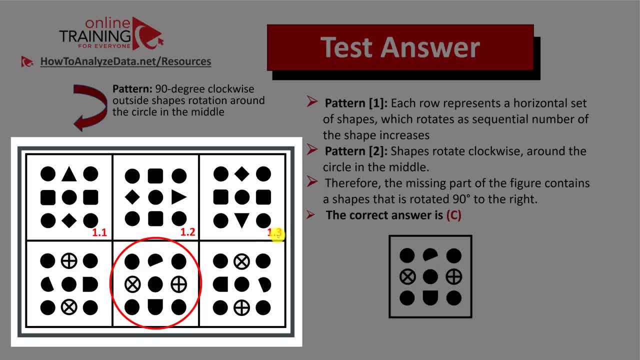 And the third shape is the first row, shape 3.. Similar pattern will exist for the bottom row. Now let's look at the pattern 2.. And pattern 2 represents 90 degree clockwise outside shape rotation around the circle in the middle. 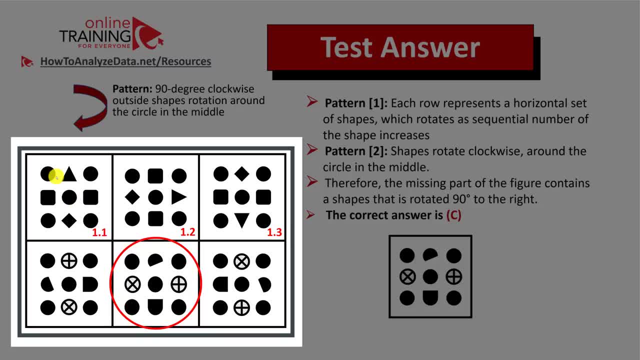 As you can see, there is always a circle in the middle And the outside shapes rotate around this circle, So let's follow the triangle. Let's look at the first shape. Here, triangle points to the top. In the next shape, triangle rotates 90 degree clockwise and points to the right. 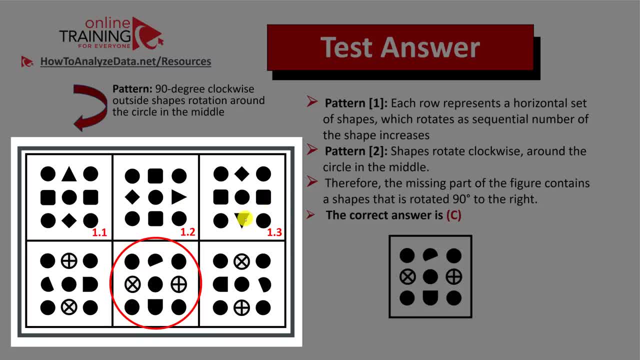 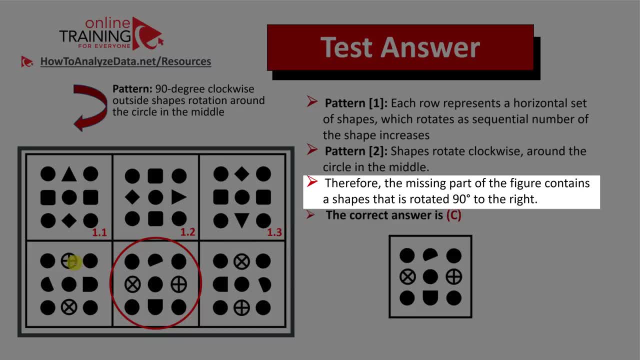 In the following shape triangle rotates another 90 degrees and follows to the bottom. Very similar pattern will exist here in the bottom row. Therefore, the missing part of the figure contains the shapes that rotate 90 degrees to the right. So the correct answer here is choice C. 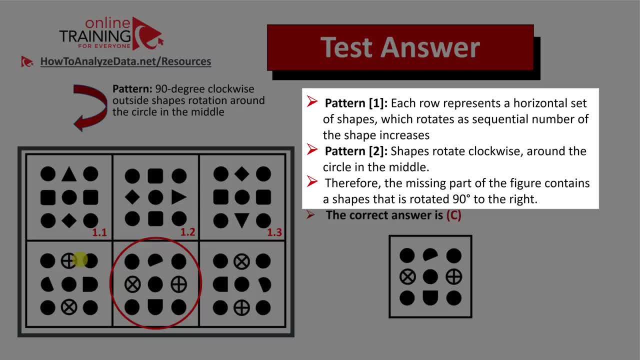 Let's recap. There are two patterns here in this question. The first pattern is the fact that each row represents a horizontal set of shapes which rotates as sequential number of shapes increases, And the second pattern indicates that the shapes rotate clockwise around the circle in the middle. 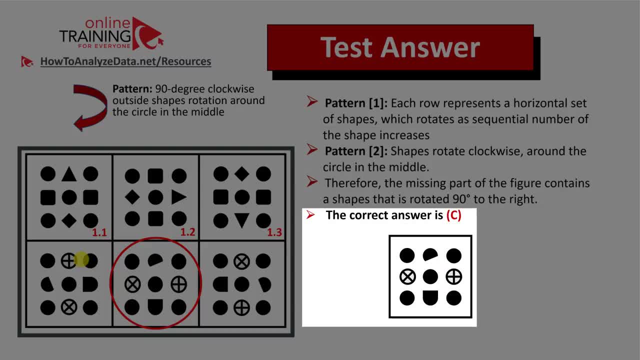 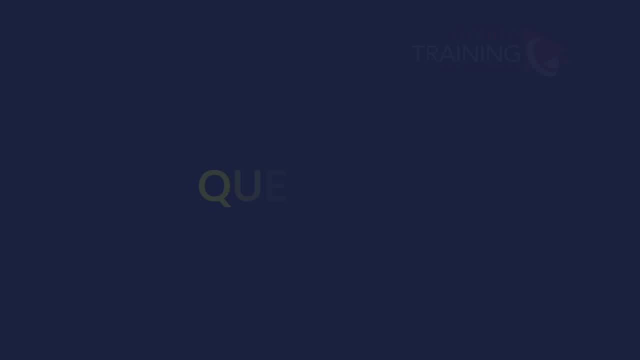 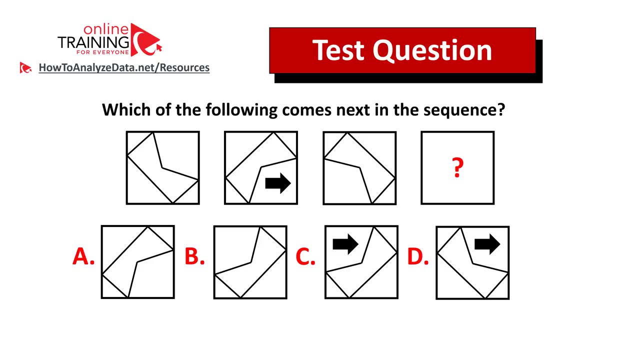 Therefore, the correct answer here is choice C. Hopefully you've nailed this question and now know how to answer similar questions on the test. Let me share with you a tricky question from the test, which validates your knowledge of pattern recognitions and logical reasoning. 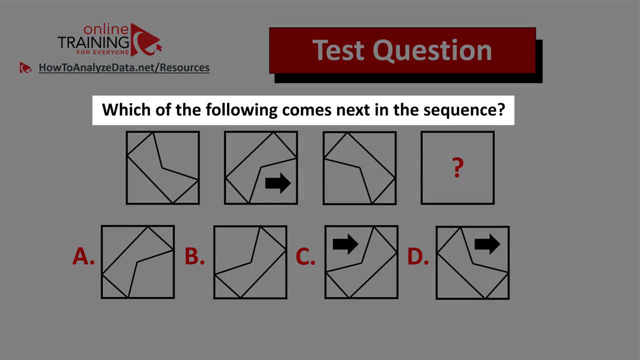 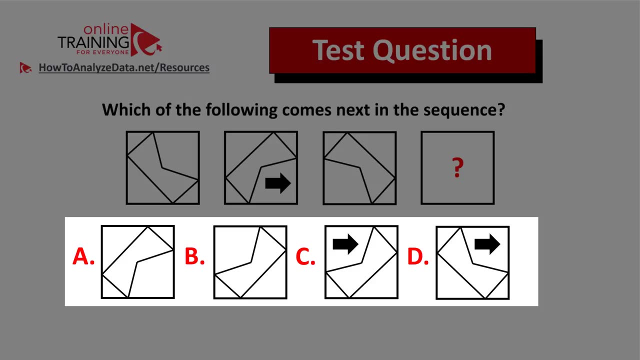 Which of the following comes next in the sequence And you're presented with four squares. The fourth square has a question mark, which means that you need to figure it out, And you have four different choices: Choice A, B, C and D. 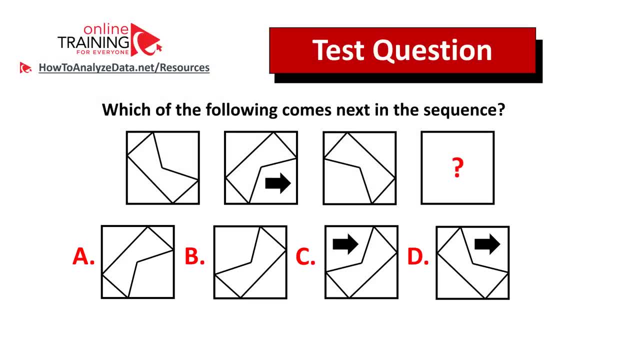 An answer is not obvious, but I'm pretty sure you will figure it out. Please give yourself 10 to 15 seconds to see if you can see the answer, Or maybe you can come up to the answer. Did you figure out the solution? 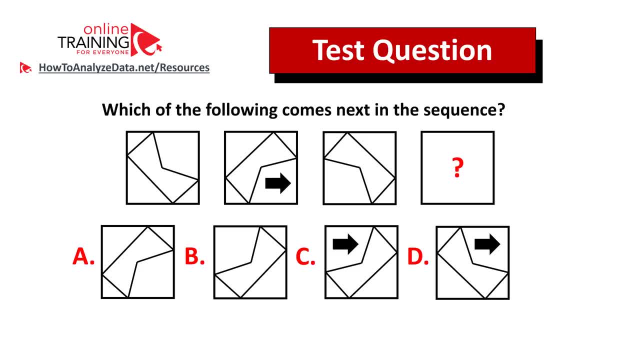 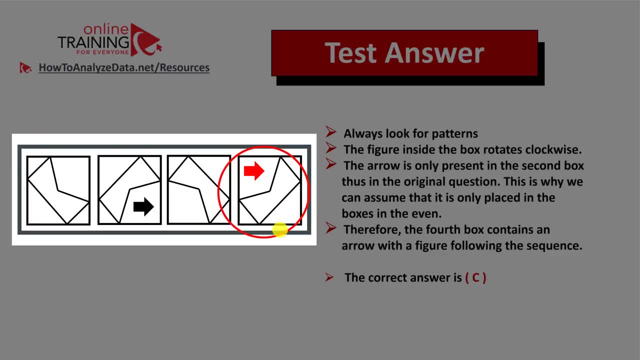 Let's continue to see how we can get to the correct solution together. And here's the answer. The fourth box in the sequence is now populated, But let's go through the logic and rationale so you would know how to answer similar questions on the test. 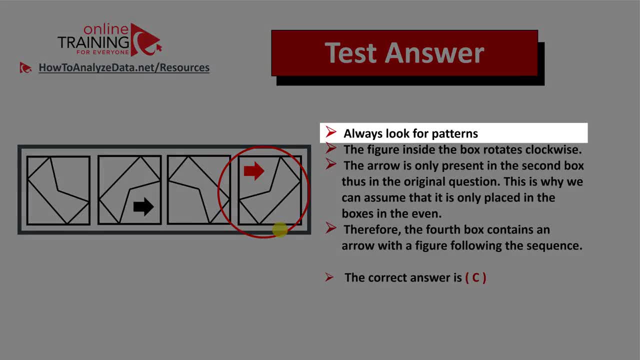 Number one tip- and always a tip- is: always look for patterns. So what you see is that the figure inside rotates clockwise. If you look at the corner of the shape, you will see that the corner was on the particular side of the square. 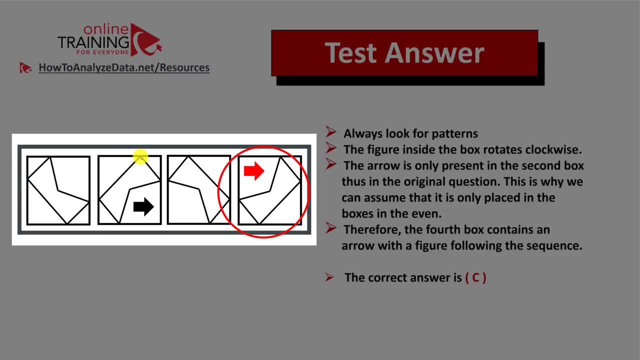 It was on the left side. Now the same corner touches the top line of the square, And then in the third box it touches the right line of the square, Which means that you can logically assume that in the following, in the fourth box, 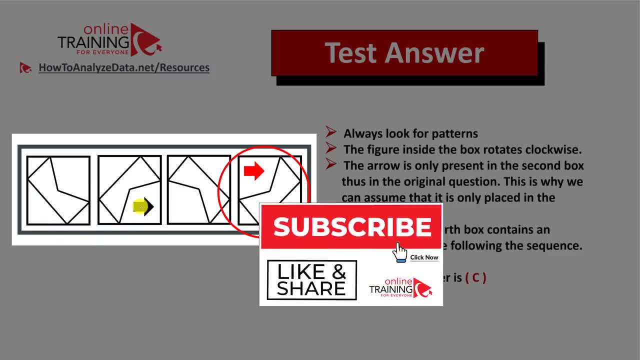 it will be touching the bottom line. There is also a pattern of arrows. You see that the box number two has the arrow pointing to the right, And boxes one and three do not have this arrow, So the arrow only present in the second box. 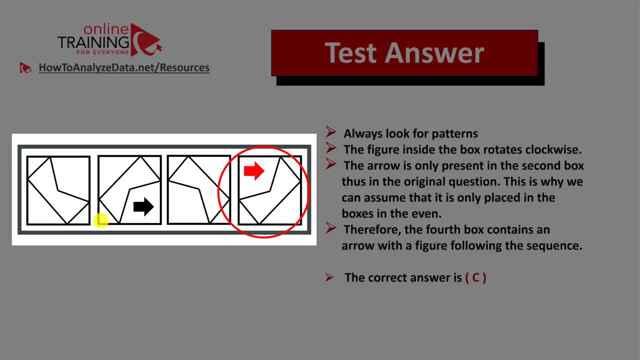 In the original question arrow is only present in the second box. We can logically assume that it only placed in the boxes that are. even Number four box is missing, So you can logically assume that the arrow should be present in the box number four. 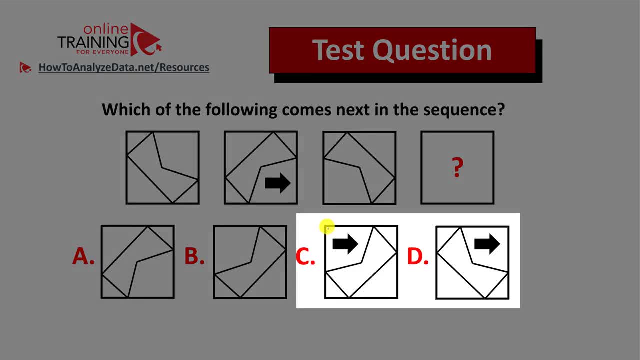 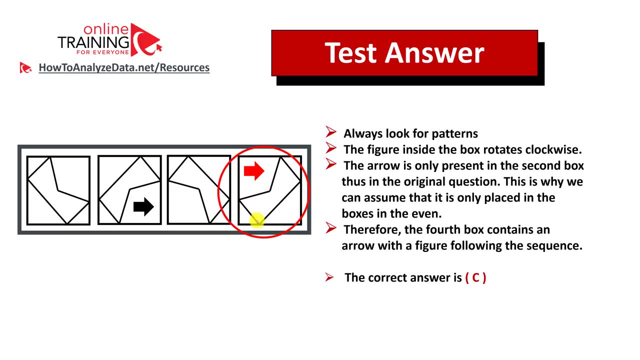 Among the choices presented, only choice C and D are valid, because only they contain the arrow And you need to determine the final box based on the position of the shape inside the square. So the correct answer here is choice C. Hopefully you've nailed this question. 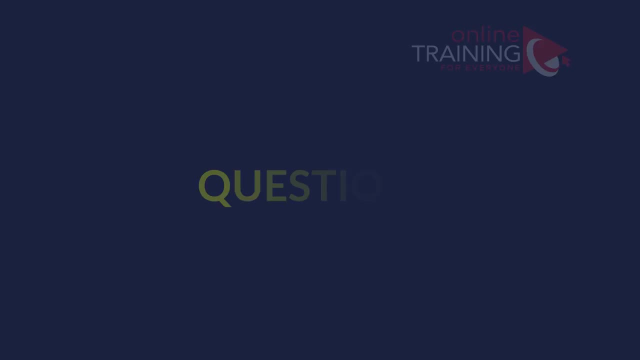 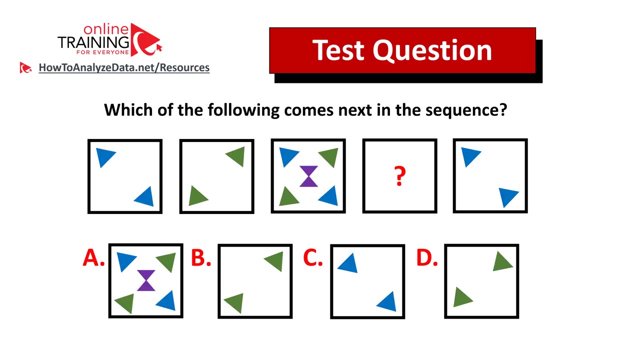 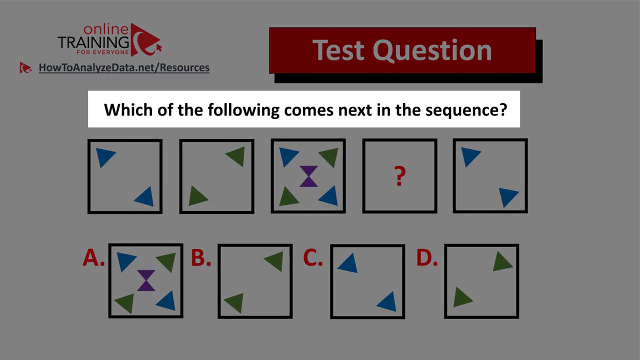 and now know how to answer similar questions in the test. Here's an interesting question which tests your knowledge of pattern recognition, logical reasoning as well as analytical skills. Which of the following comes next in the sequence? You're presented with the sequence of five shapes. 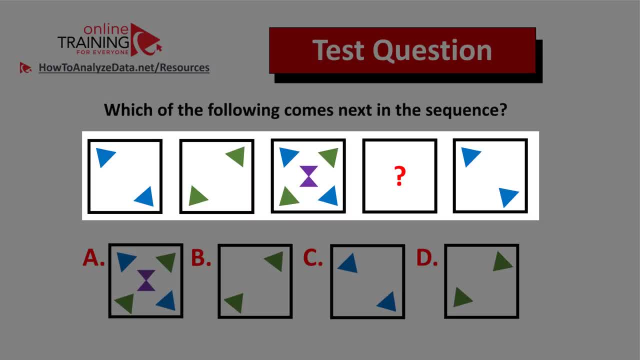 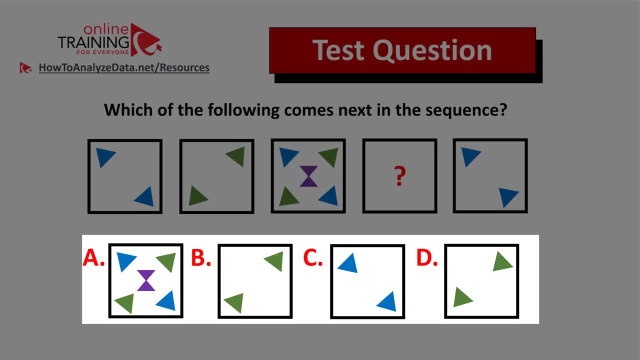 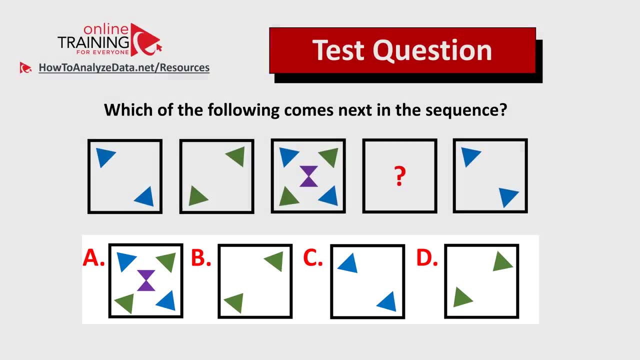 five squares which have triangles. inside, One square is missing triangles And you would need to make a selection. which square is missing out of four possible choices- Choices A, B, C and D? An answer here, believe me, is not obvious. 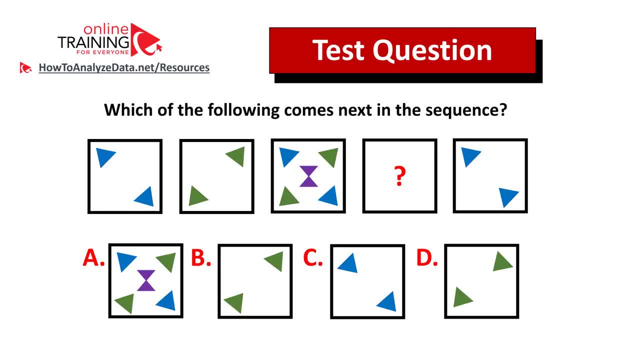 Give yourself 10 to 15 seconds to see if you can recognize the pattern and come up with the answer. Did you figure out the solution? Let's continue to see how we can solve this challenge and get to the correct solution together. Typically, there are patterns. 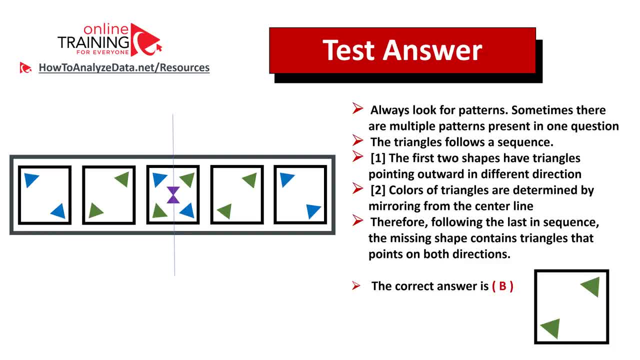 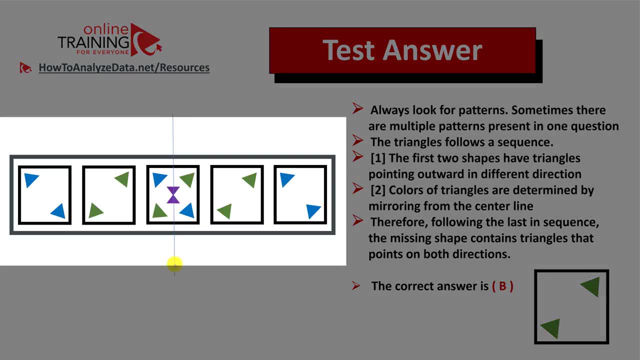 on the test questions. What you need to do to find out the right answer is to recognize the patterns. There are multiple patterns in this question. Pattern number one is that the first two shapes have triangles pointing outward in the different directions, And you also see this is the mirror line. 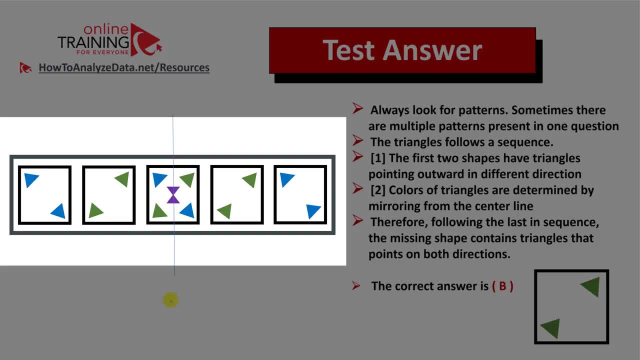 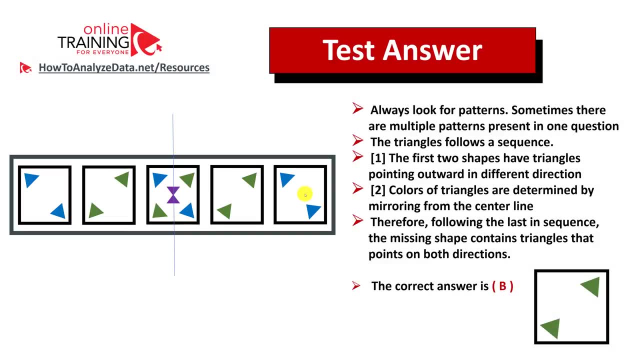 And then from the mirror line, you see that the colors go in a different pattern: Green and blue to the left. So the same thing should happen from the mirror line to the right: Green and blue. Therefore, this is why the missing shape. 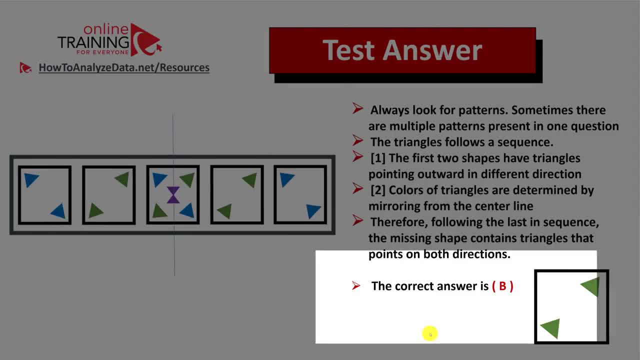 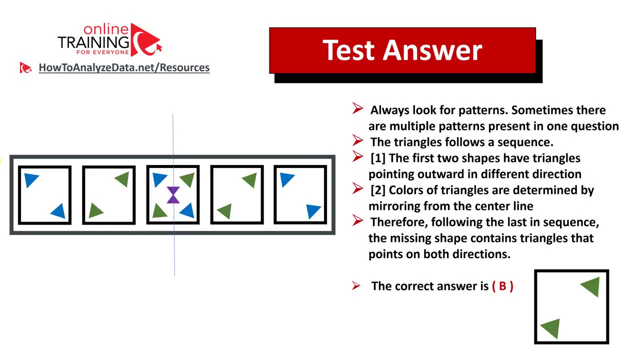 will contain green triangles that point in both directions. So the correct choice here is choice B. Hopefully you've nailed this question and now know how to answer similar questions in the test. And now here's the question for you to try If you figured out the answer. 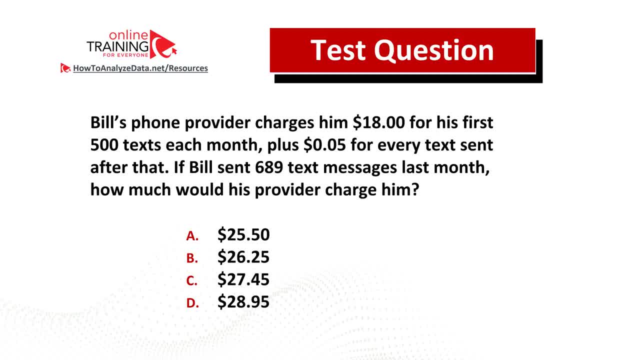 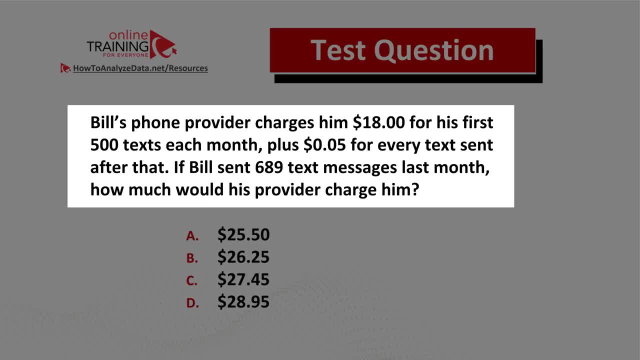 please post it in the comments of this video so I can give you my feedback. Bill's phone provider charges him $18 for the first 500 texts each month, plus 5 cents for every text sent after that. If Bill sent 689 text messages last month, 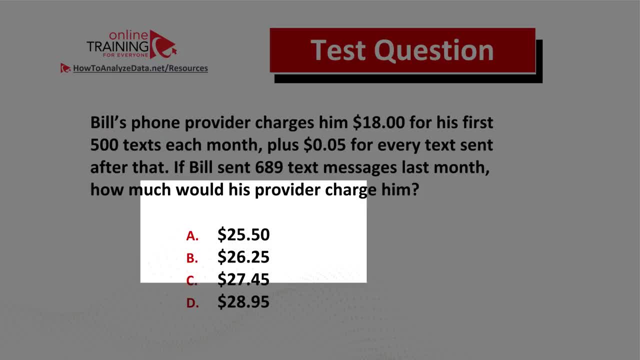 how much would his provider charge him? And you're presented with four different choices: Choice A: $25.50.. Choice B: $26.25.. Choice C: $27.45.. And choice D: $28.95.. You can pause this video. 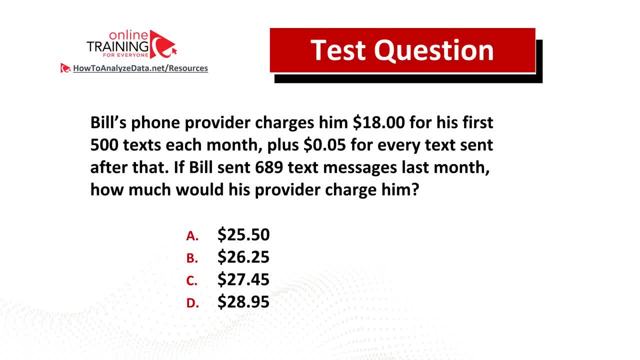 and try to solve this challenge now And if you have figured out the answer, feel free to post the answer in the comments section of this video, along with your rationale, so I can give you my feedback. I'm also planning to post a detailed answer. 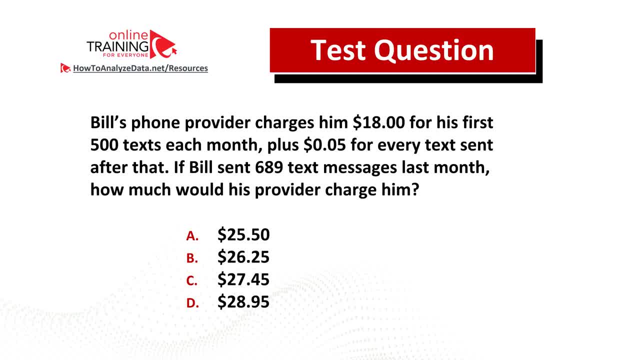 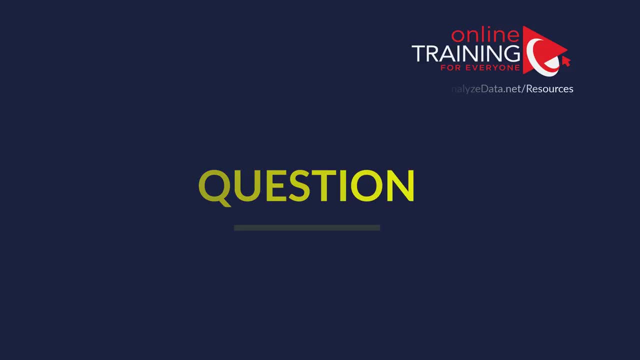 in my future videos, so make sure to subscribe and review my latest videos on the topic to learn about the answer and how to come up with the answers to similar questions in the test. Thanks for participating and good luck. Here's the tricky question to test your pattern recognition skills. 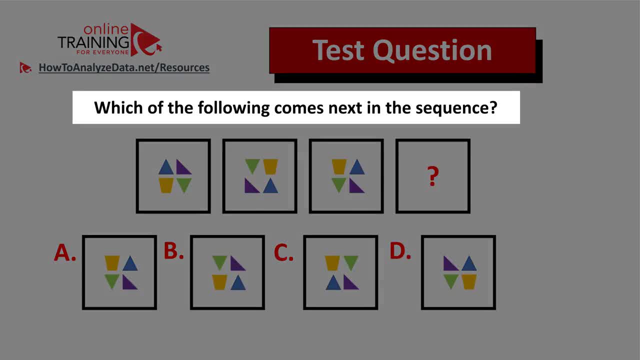 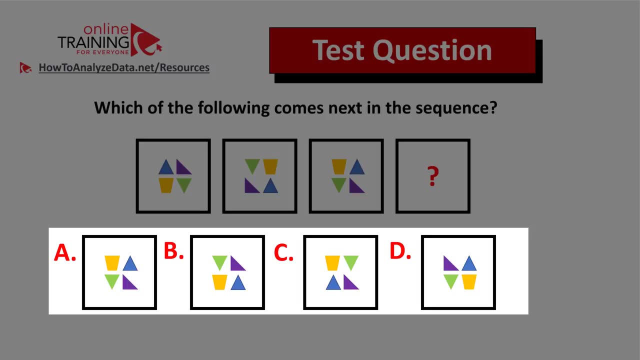 Which of the following comes next in the sequence, And you're presented with the sequence of five squares. Each square has smaller shapes inside. The fourth square is unknown and you need to detect it from the four possible choices: Choice A, B, C and D. 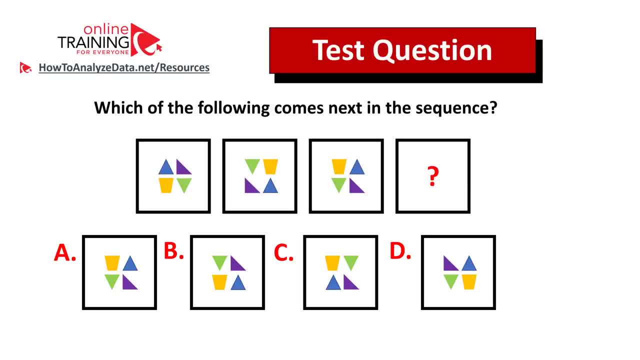 Do you see the answer? It's not obvious. Give yourself 10 to 15 seconds to see if you can recognize the answer. Did you figure out the solution? Let's continue to see how we can solve this challenge and get to the correct solution together. 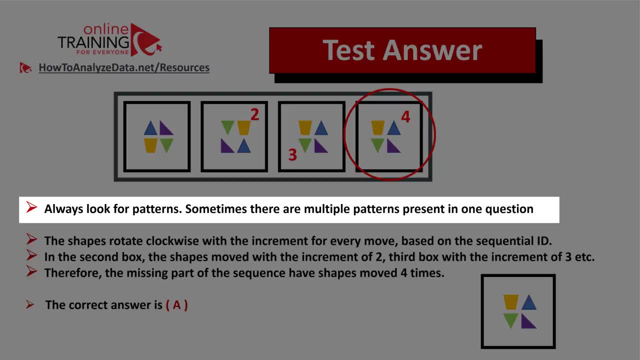 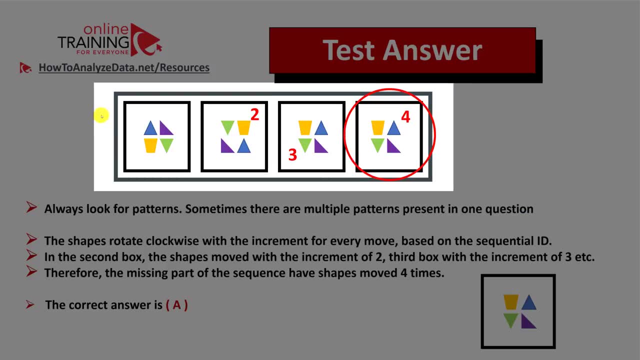 As usual, always look for patterns. A lot of times there are multiple patterns present in the question, but in this particular case, there is only one pattern, And the pattern is is that the shapes rotate clockwise, with the increment on every move. 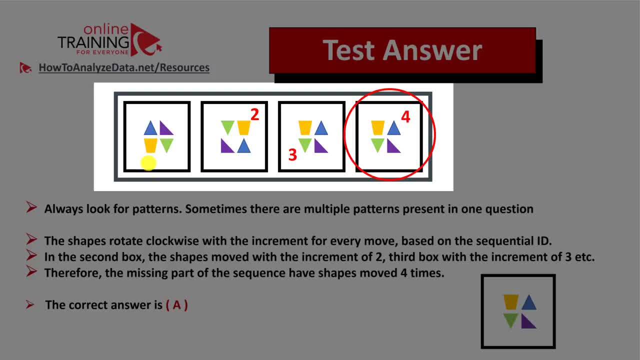 For example, if we look at the shapes going from box number one to box number two and we follow the yellow shape, we will see that it moved from the position at eight o'clock to the position at two o'clock. And this happens because they move one from box one to box two. 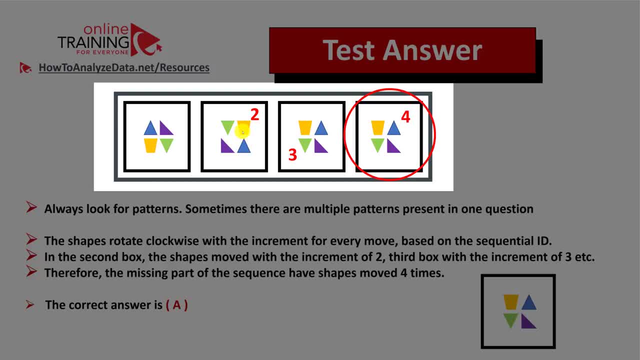 So the next increment, if we follow the same yellow box, would be with the increment of three, If we do the math one, two and three, and that would determine the next position of the yellow box, And this is yellow box. 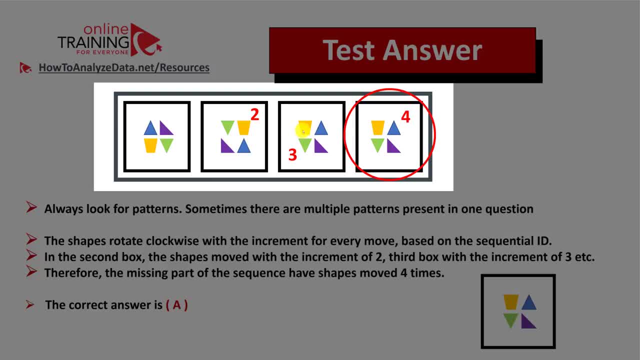 in the square number three. If we follow this pattern logically, you will see that the next move in the shape number four would be one, two, three, four, basically coming back to the same position. Tricky question, but the answer is easy. 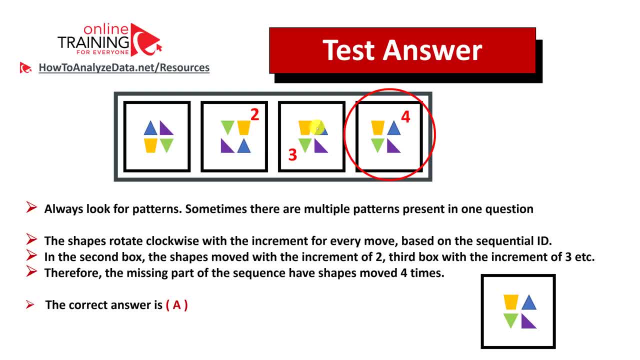 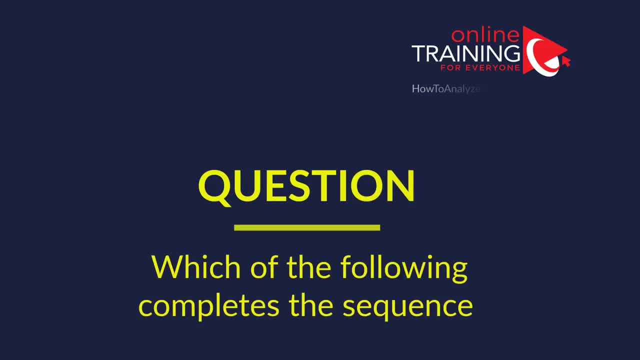 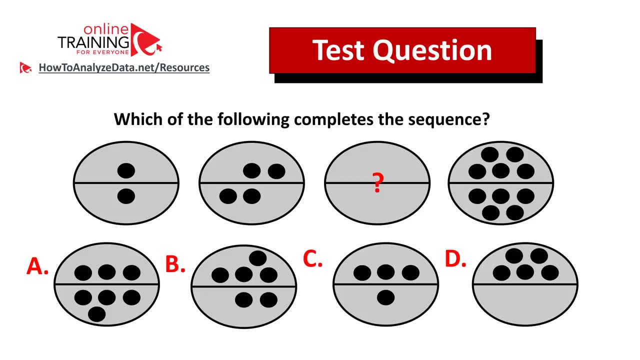 as long as you know the pattern. Hopefully you figured out the answer and now know what to look for in similar questions in the test. Let me share with you a tricky question which tests your analytical and pattern recognition skills. Here is the question: Which of the following? 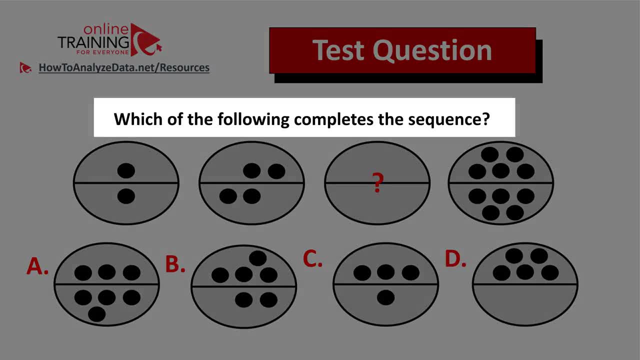 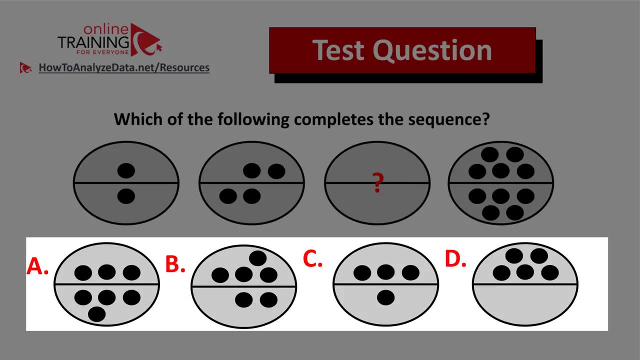 completes the sequence. You are presented with the sequence of four or more, or four ovals, and the third one is missing, And you have four different choices to choose from: Choice A, B, C and D, All choices with the similar ovals. 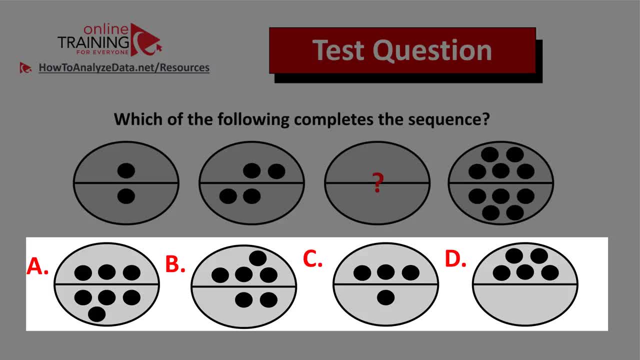 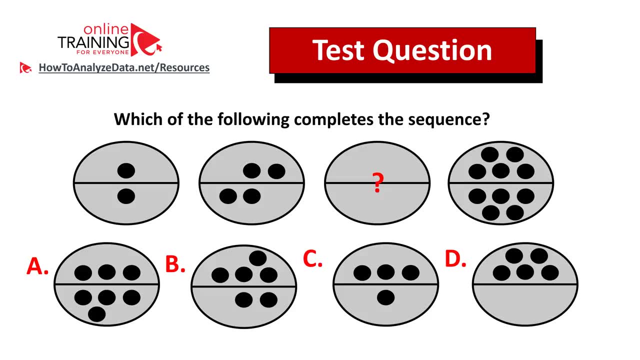 just with the different dots located in the different places of the oval. Do you think you see the answer? Take a look carefully and maybe spend 10 to 15 seconds looking at this particular question, possibly stopping the video. Did you figure out the answer? 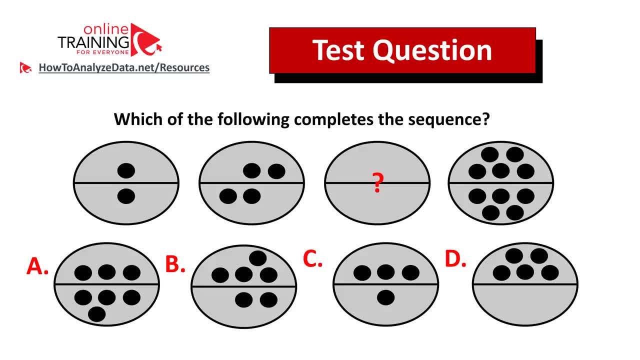 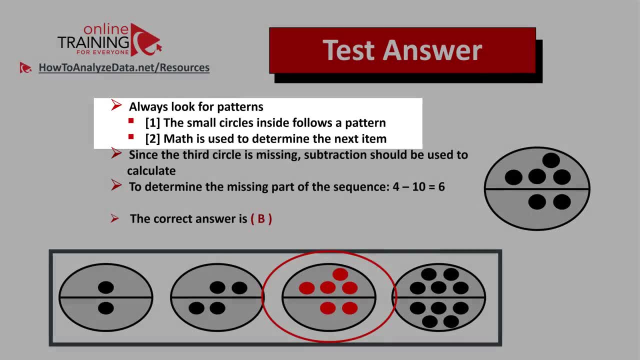 Let's continue to see how we can get to the correct solution together. When solving any type of questions, always look for patterns, And if you look carefully, you will see multiple patterns happening here. The first pattern is: there's always a small circle. 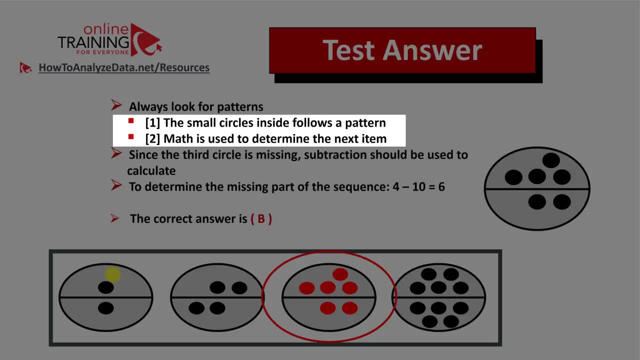 inside the larger oval. And then the second pattern for this particular question is that the math is used to determine the next item. And since math is used, we can use calculations to determine the missing part. You see that the item number two has four small circles. 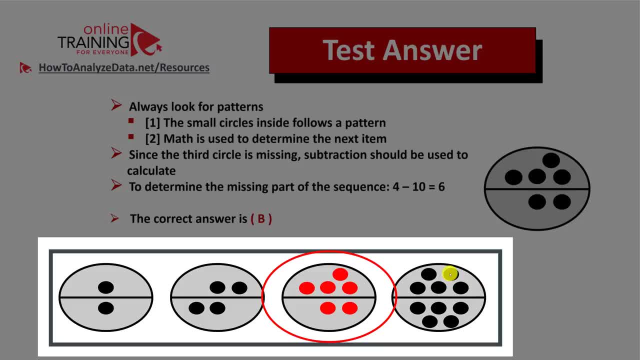 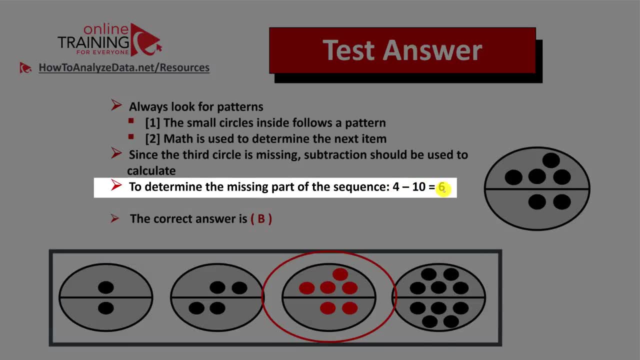 And the item number four has 10 small circles. So we can use subtraction to calculate the item in the middle, And if we subtract 10 minus four we will get to six. So the correct answer here is choice B. Hopefully you've nailed this question. 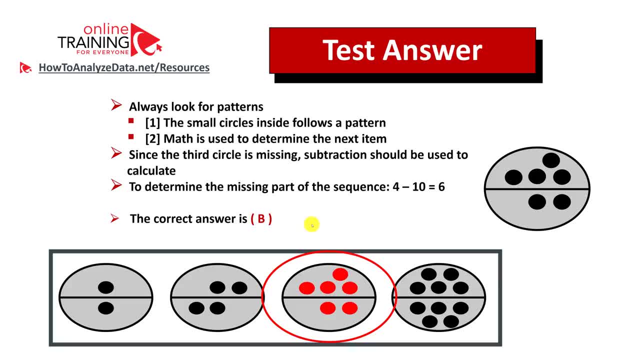 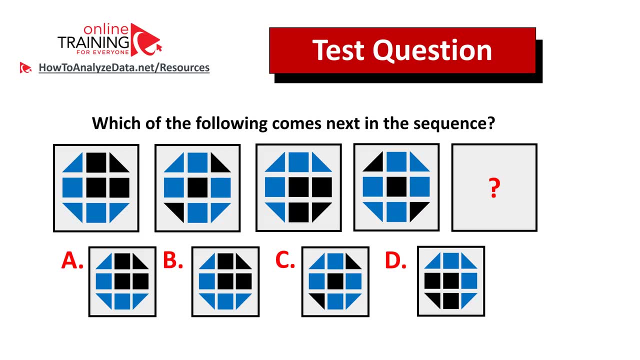 and now know how to answer similar problems in the test. But in case you need more practice problems, please check out my ebook in the description section of this video. Thank you. Let me share with you a tricky question from the real test. Somehow, though, 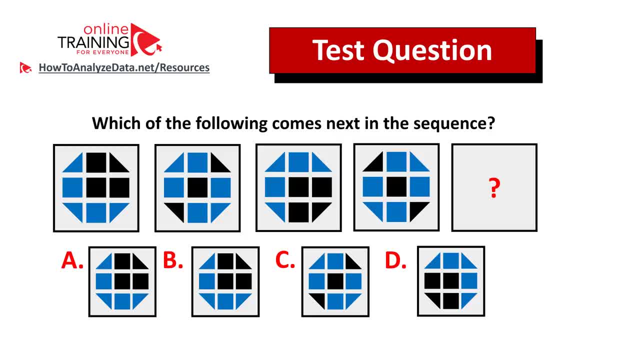 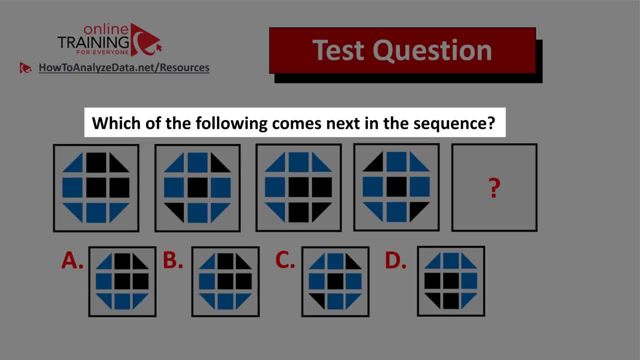 I have a confidence that you will figure out the answer, especially if you will closely look for patterns. Here's the question: Which of the following comes next in the sequence? You're presented with the sequence of four squares, and fifth one is missing. 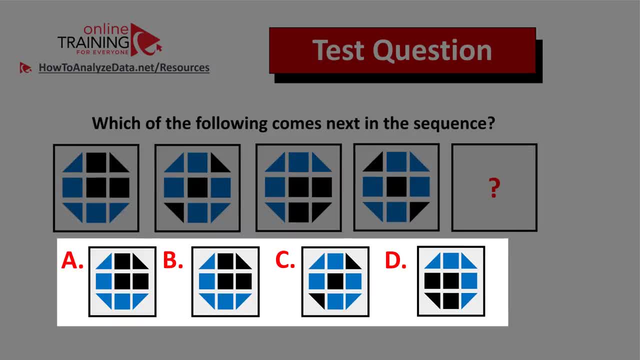 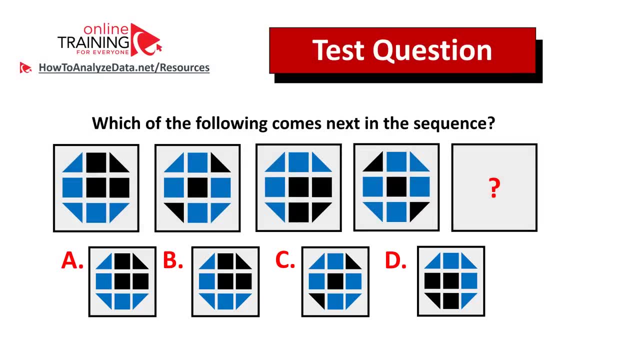 And obviously there are four possible choices- Choices A, B, C and D- And all of these choices look very similar. Do you think you know the answer? Now might be a good time to pause this video and give yourself 10 to 20 seconds. 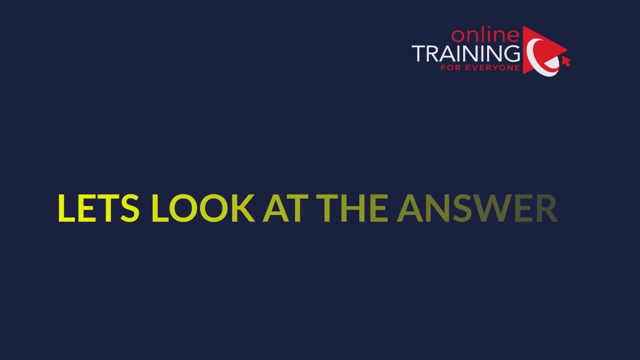 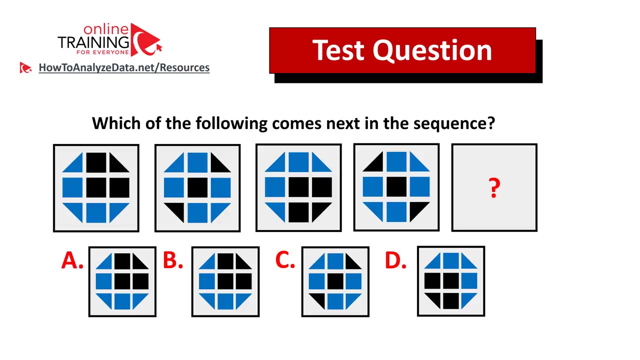 to see if you can come up with the answer. Did you figure out the pattern? Do you think you know the answer? Let's continue to see how we can solve this challenge together. As usual, my advice to you: always look for patterns. 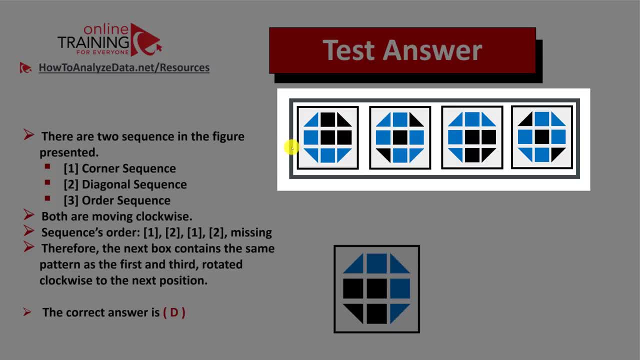 And if you look closely you see that there are at least three different patterns presented here. There is a pattern for corner sequence. This is the boxes, for example, here in the upper right corner, And they move clockwise. You see the pattern continues in the box three. 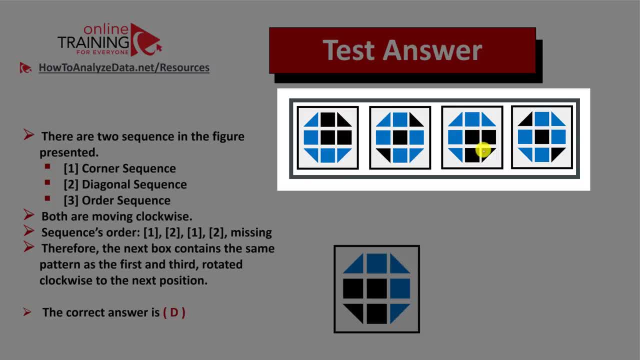 And the upper right corner becomes bottom right corner. There is also a diagonal sequence And I show this sequence right here in the boxes two and four, And diagonal sequence also moves clockwise. It moves from the top right corner to the bottom left corner. 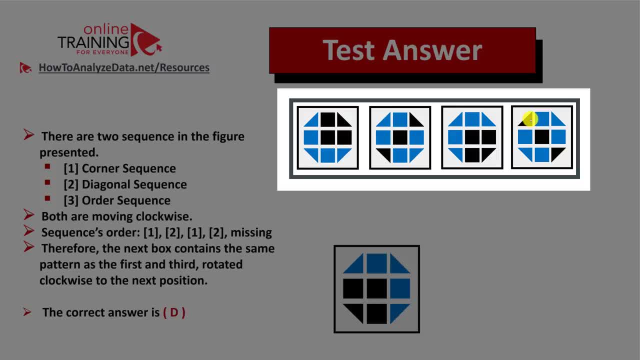 And in the box four it goes from the upper left corner into the bottom right corner. So once you know both sequences, you can calculate the missing item number five, And the logic here is that the next box will contain the same pattern as the first. 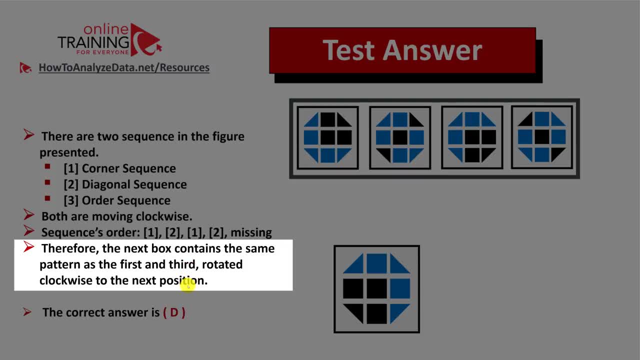 and the third rotated clockwise to the next position. Let's recap. There are two sequences in the figure presented. We have corner sequence, we have diagonal sequence and order sequence. Corner sequence goes in boxes one and three and diagonal sequence goes in boxes. 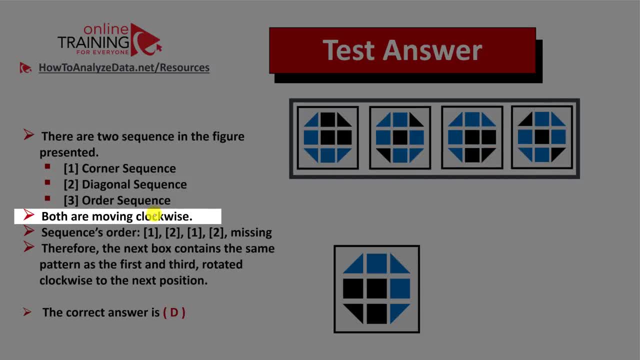 two and four. Both sequences move in clockwise in the next item And the sequence's order is one, two, one, two and then the missing item. This is why the next box will contain the same pattern as the first and the third. 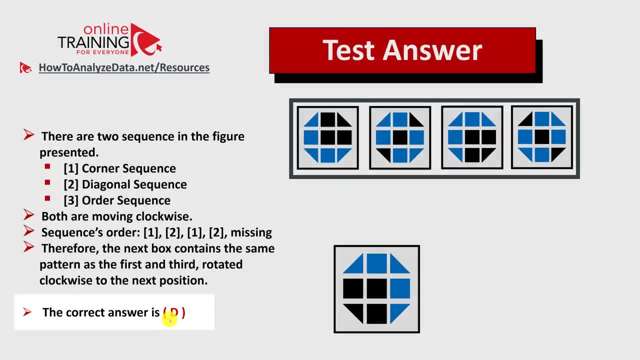 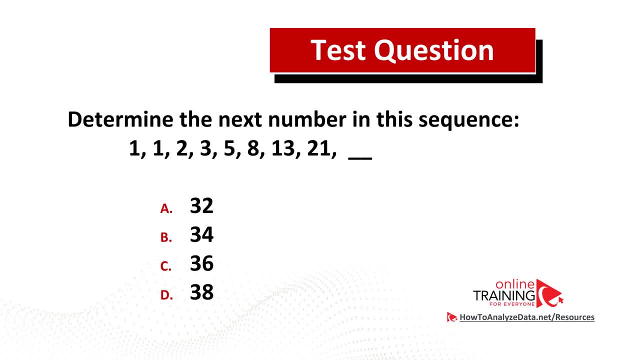 rotated clockwise to the next position. So the correct choice here is choice D. Hopefully you've nailed this question. Here is the question from the real test you can try to solve on your own. I have full confidence that you can solve this challenge from the real test. 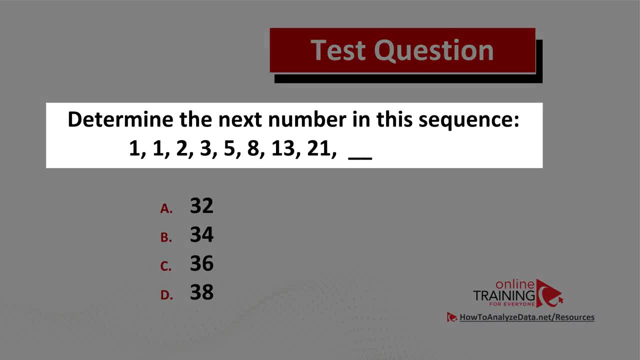 Determine the next number in this sequence, And you have a series of numbers presented on the screen: One, one, two, three, five, eight, 13,, 21, and then the missing number that you need to figure out. You have four choices. 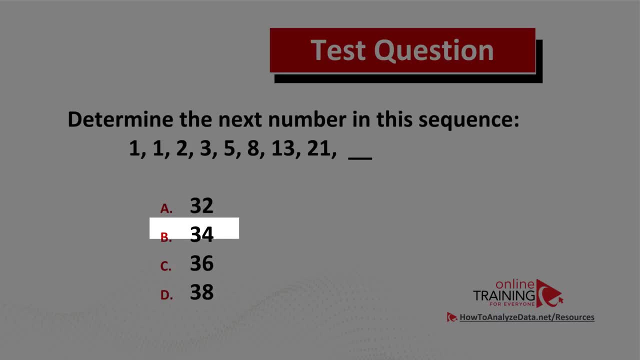 to pick from Choice A: 32., Choice B: 34., Choice C, 36. And Choice D: 38.. Feel free to pause this video and try to solve this challenge now, And if you have figured out the answer. 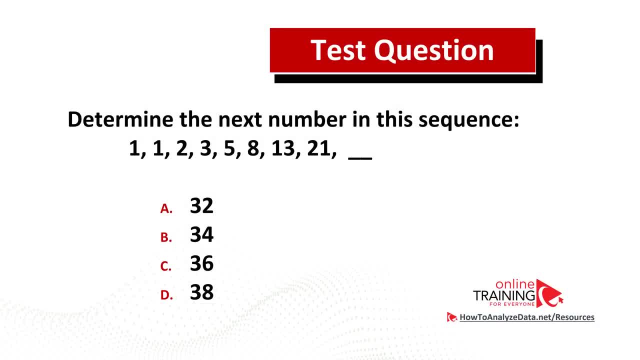 feel free to pause the answer in the comment section of this video. Please also include your rationale so I can give you my feedback. I am also planning to post a detailed answer in my future videos, so make sure to subscribe and review my latest videos. 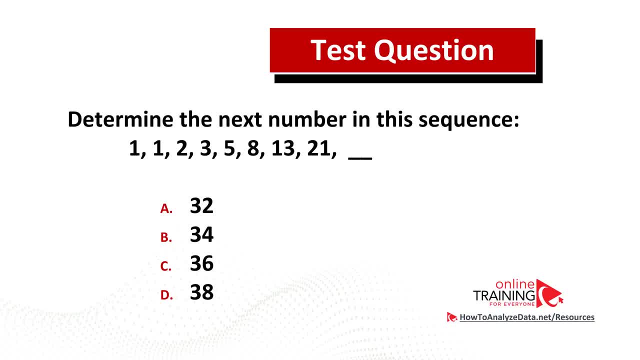 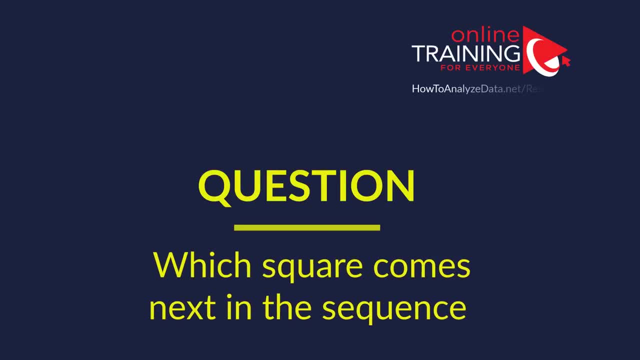 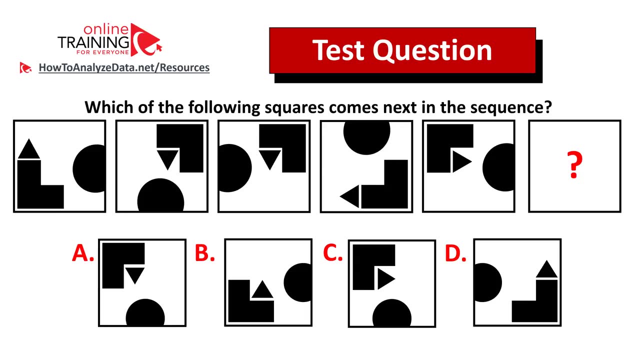 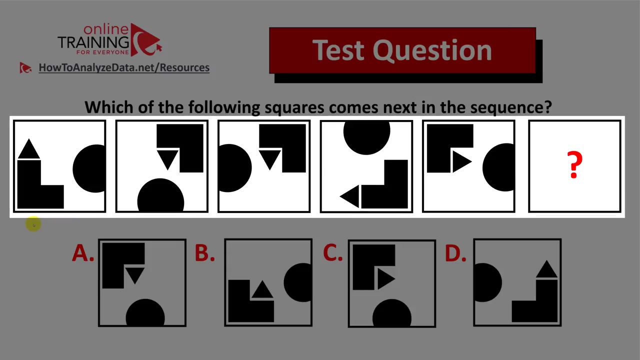 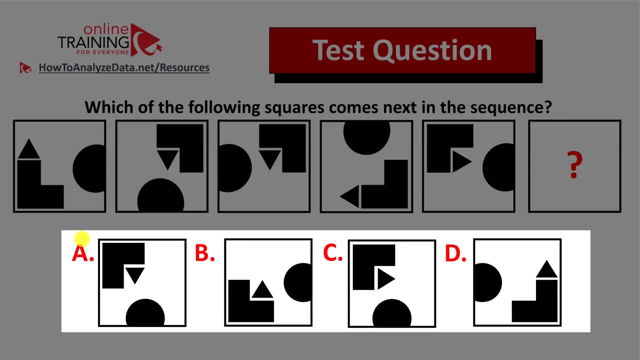 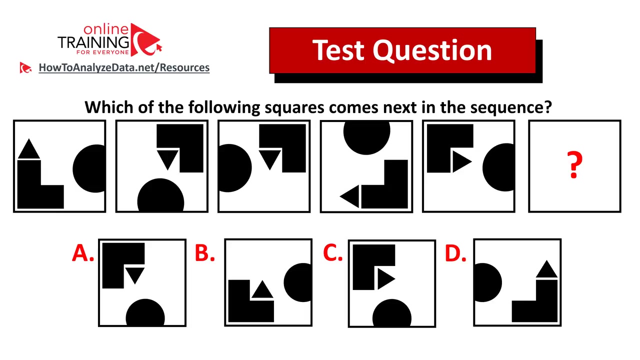 on the topic to learn about the answer and how to come up with the answers to similar questions in a test. Thanks for participating and see you in the next video. Bye-bye, Give yourself 10 to 15 seconds to look closely and see. 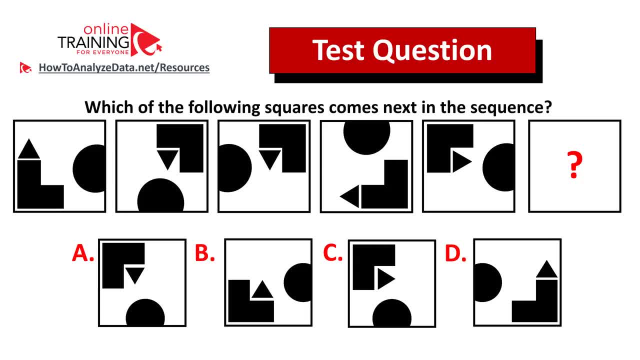 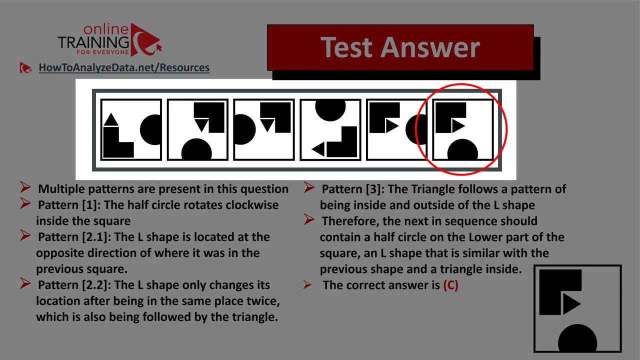 if you can recognize which shape should be selected out of the four choices presented. Did you figure out the solution? Let's continue to see how we can get to the correct answer and solve this challenge together. As usual, my recommendation to you is always: 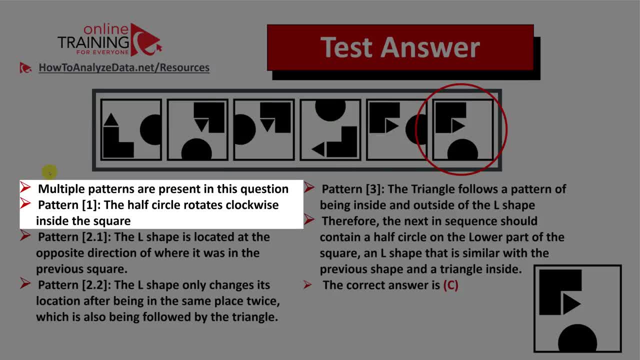 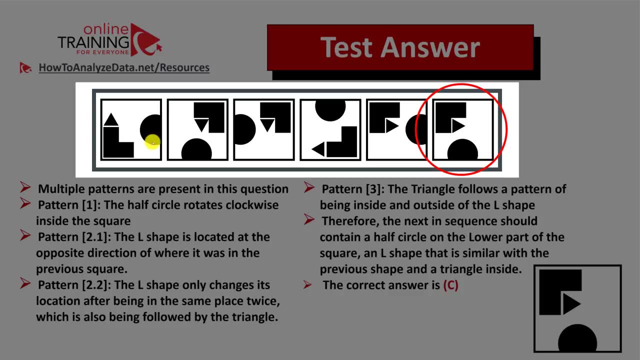 look for patterns And let me share with you which patterns are present in this question. The first pattern is where half circles rotate clockwise inside the square. So the first position is on the right, next position is at the bottom, then left top. 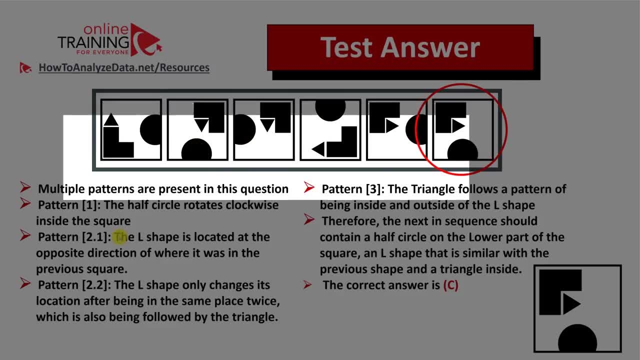 and then you see the cycle repeating. The second pattern is where L shape is located at the opposite direction of where it was in the previous square. So you see that the L shape in the first square is located in the bottom left In the next square. 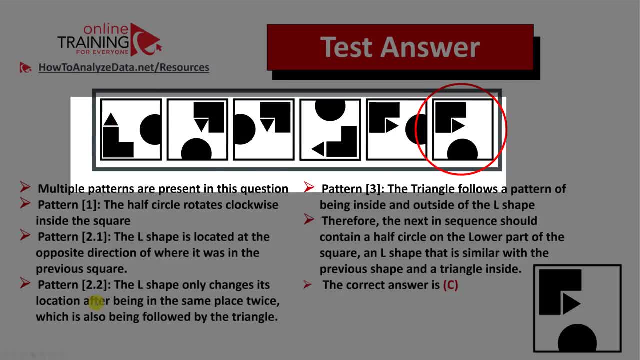 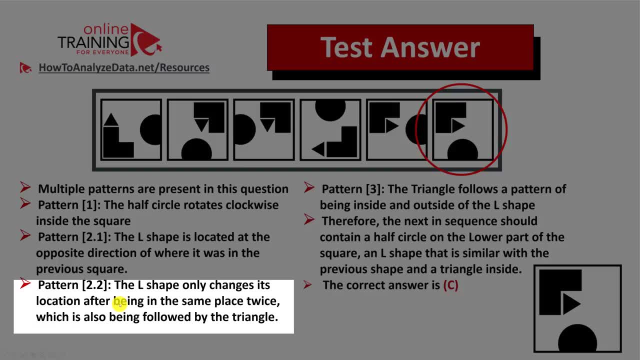 it's located in the upper right corner And the next square is located in the upper left corner. Then the third pattern, also related to the L shape, is where L shape only changes its location after being in the same place twice, which is also being followed. 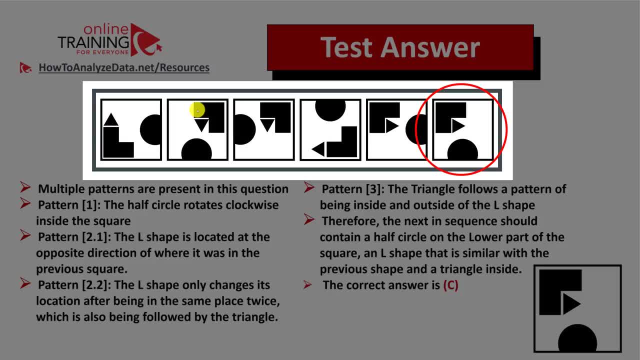 by the triangle. As you can see, the L shape in the first square is located in the bottom left corner, And then in the next two shapes it's located in the upper right and then in the upper right again. Then it changes the position and goes. 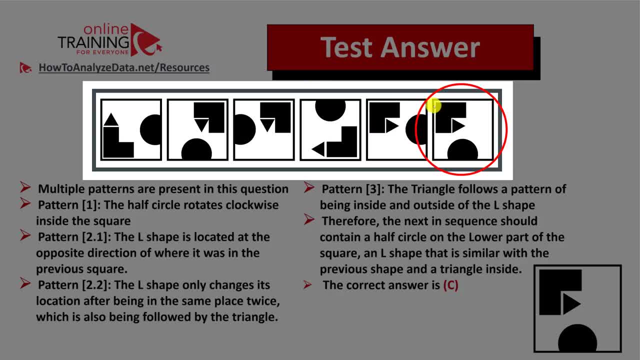 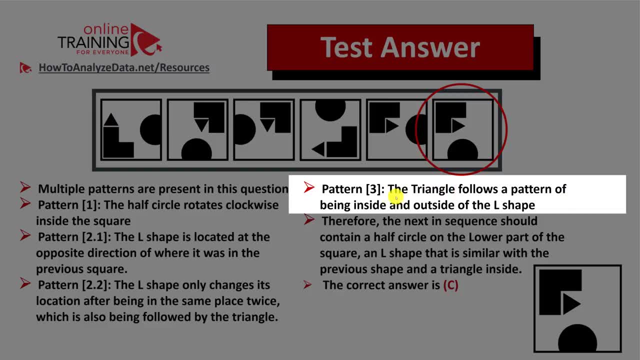 into the bottom right, And then the next two positions are located in the upper left again, And then the last but not least pattern is the pattern of the small triangle, And small triangle here follows the pattern of being inside and outside of the L shape. 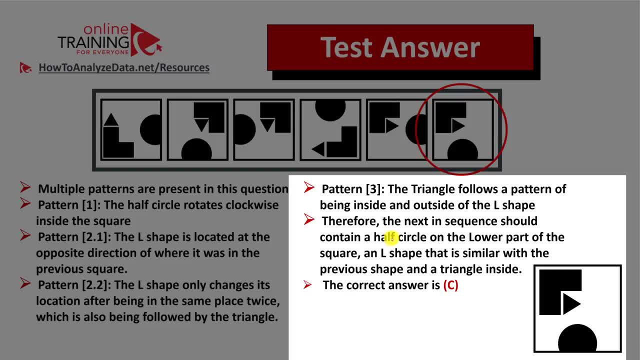 Therefore. this is why the next item in the sequence should contain a half circle in the lower part of the square and then the L shape, which is similar with the previous shape, and the triangle inside. So the correct answer is choice C. Hopefully you understand what to look for. 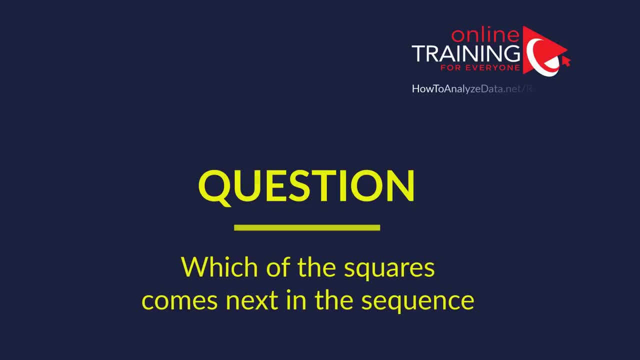 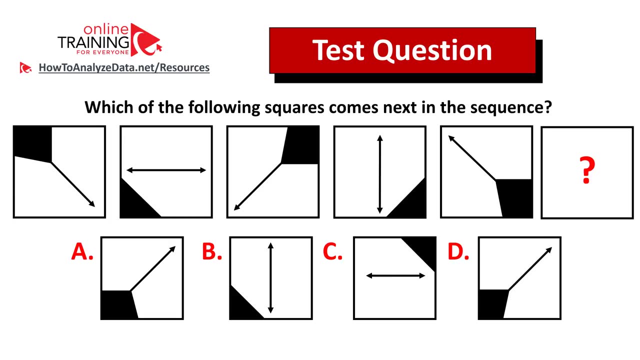 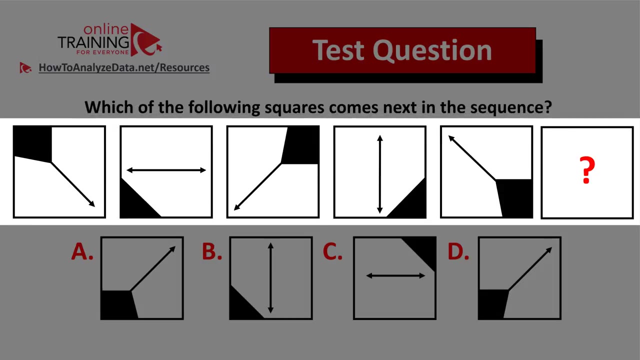 in the similar questions in the future. Let me share with you a tricky question which tests your pattern recognition reasoning as well as analytical skills. Which of the following squares comes next in the sequence? You are presented with the sequence of six squares and square number six. 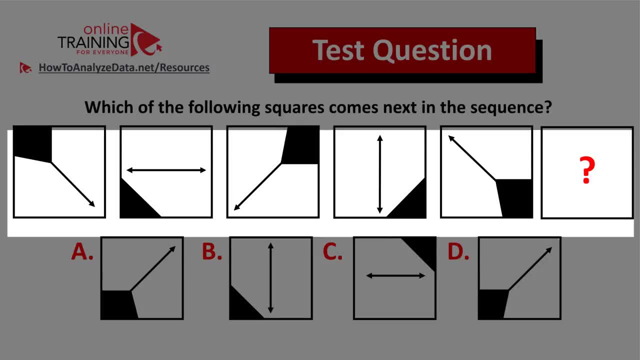 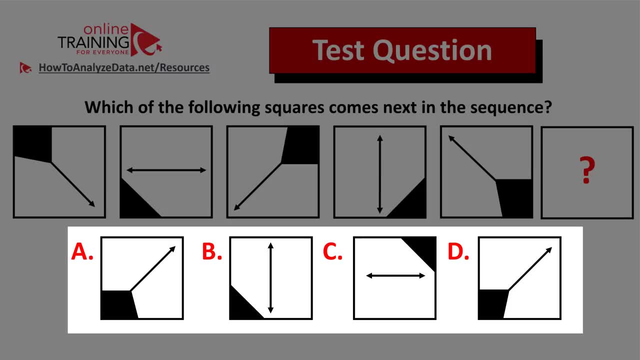 is missing And you need to pick it up. out of four different choices: Choice A, B, C and D. As always, my recommendation is look for patterns. You can pause this video for 10 to 15 seconds to see if you can come up. 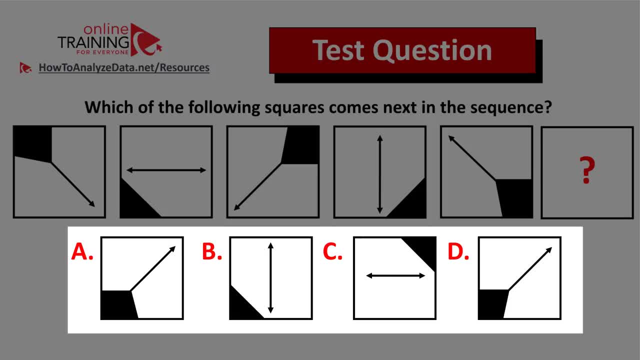 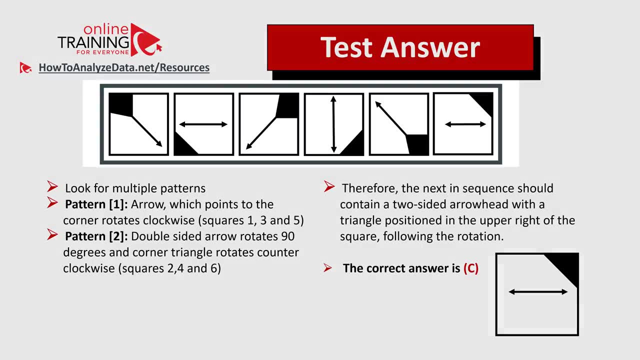 with the solution. Did you figure out the answer? Let's continue to see how we can solve this challenge and get to the correct solution together. As always, my recommendation for you is: look for patterns, And there are two key patterns present in these questions. 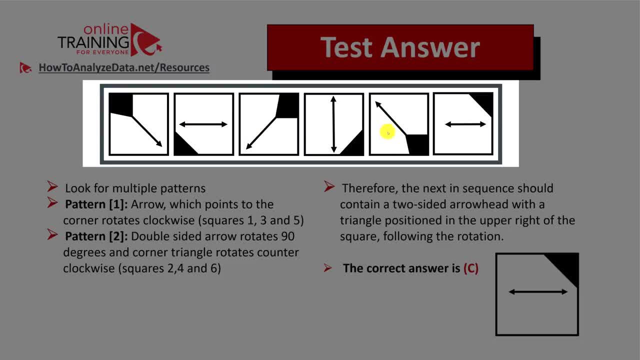 One pattern is in the squares one, three and five. What we see here? we see an arrow which rotates, and this particular arrow rotates clockwise, Specifically in the square of it arrow. So the first one is in the upper left corner, then in square number three. 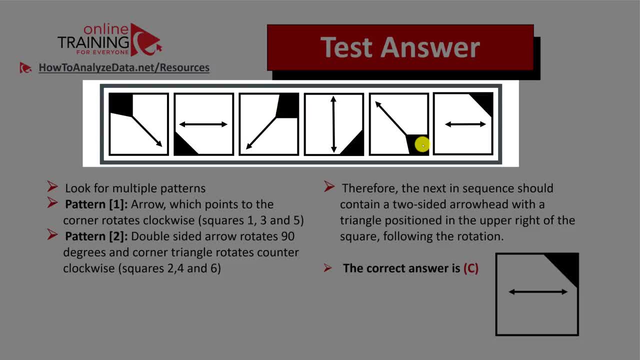 it moves into the upper right corner And then, in square number five, it moves to the bottom right corner. Then we have a completely different pattern of squares two, four and six, which was missing, And this particular pattern is double-sided. arrow rotates 90 degrees. 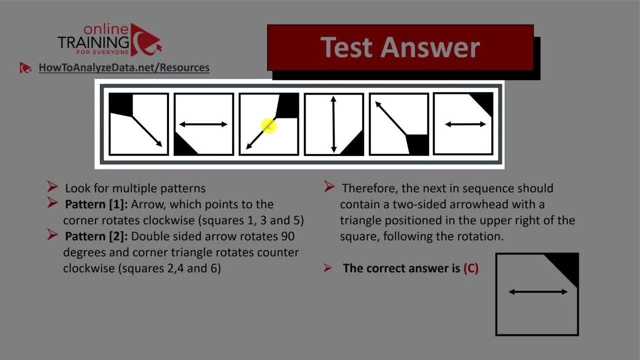 which you can see here, presented here, is completely horizontal. here it's completely vertical. So in square number six it will be horizontal again. And then another thing that happens here: the corner of the square rotates counterclockwise and it goes from the bottom left corner. 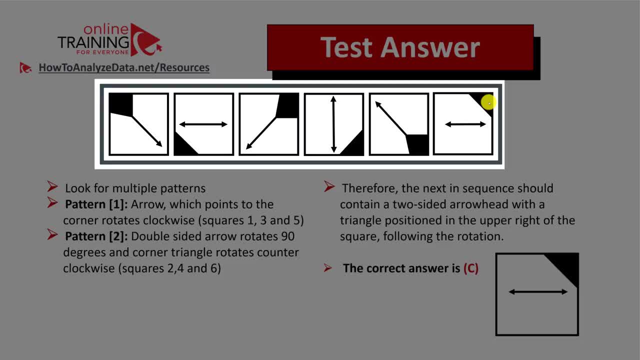 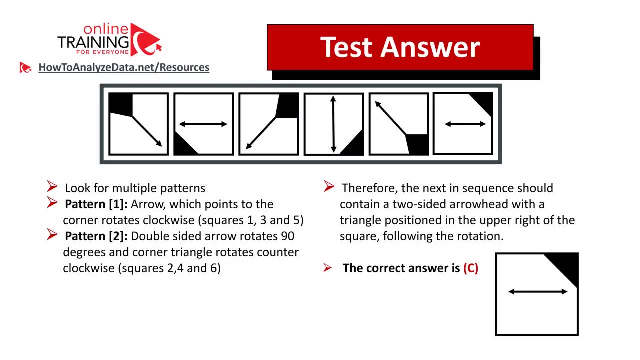 to bottom right corner. so the next position for that corner would be upper right corner. So the correct answer here is choice C. Hopefully you've nailed this question and now know how to answer similar problems on the test. Let's look at the very interesting question. 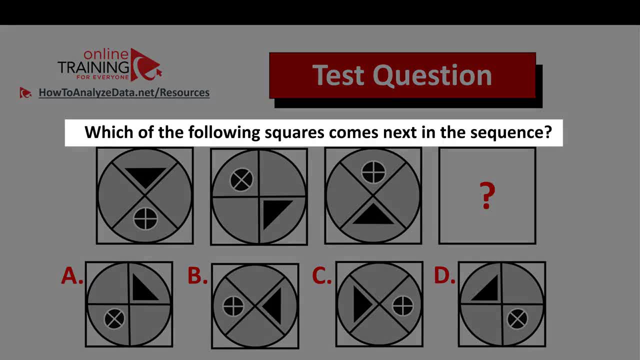 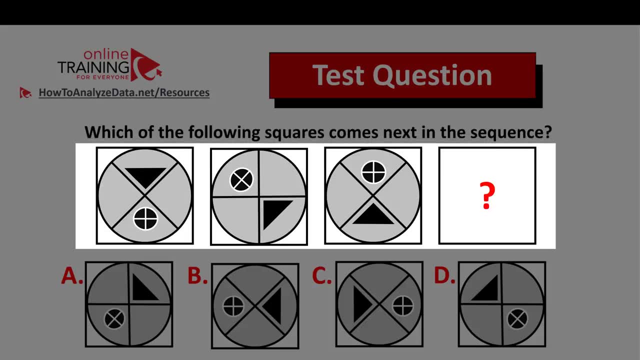 you might frequently see on the test Which of the following squares comes next in the sequence. You're presented with four squares. Each square contains a circle inside and circle has four quarters. In two of the quarters are different objects. You see triangle and you see another circle. 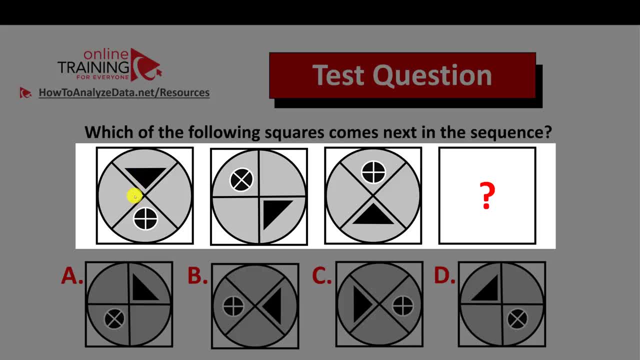 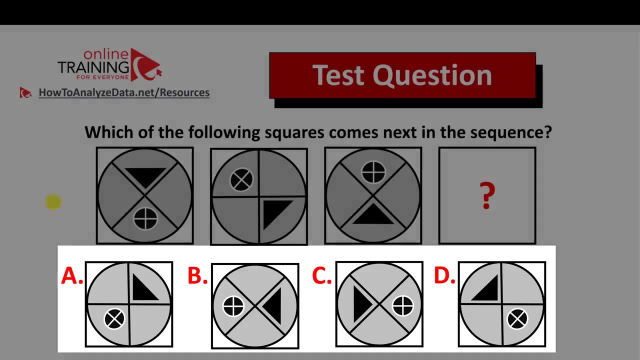 much smaller circle. You have triangles and circles, as well as quarter sections located in the different positions, and you need to determine which object comes next in the sequence. You're presented with four different choices: A, B, C and D. but first you need to understand the pattern. 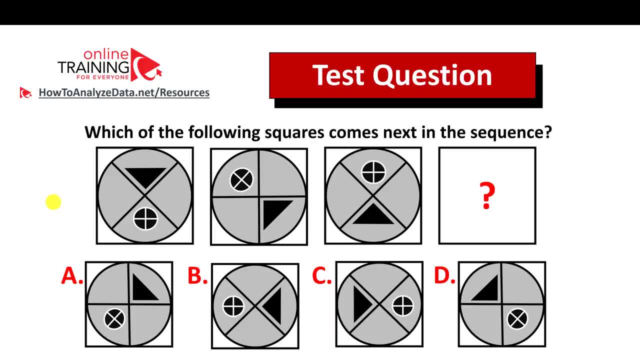 Do you see the pattern? Please give yourself 10 to 15 seconds to see if you can come up with the solution. Did you figure out the answer? Let's continue to see how we can get to the correct solution and solve this challenge together. 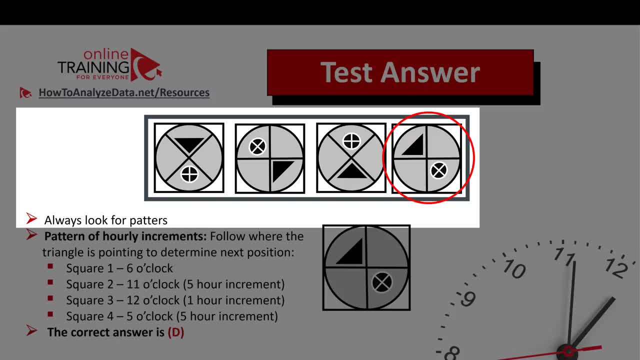 As usually, my recommendation is always look for patterns. I know sometimes it's hard to see those patterns, but you still need to keep looking. In this particular case, we're dealing with the pattern of hourly increments and we determine the hour based on where the triangle is pointing.